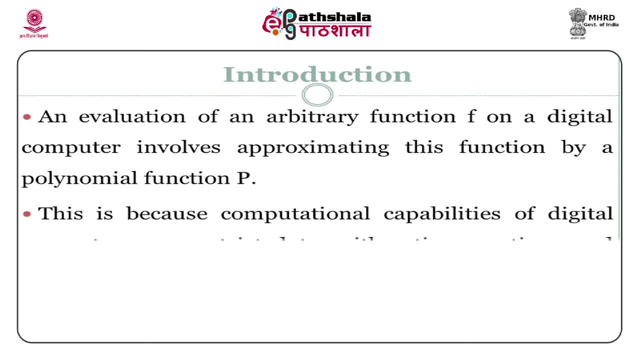 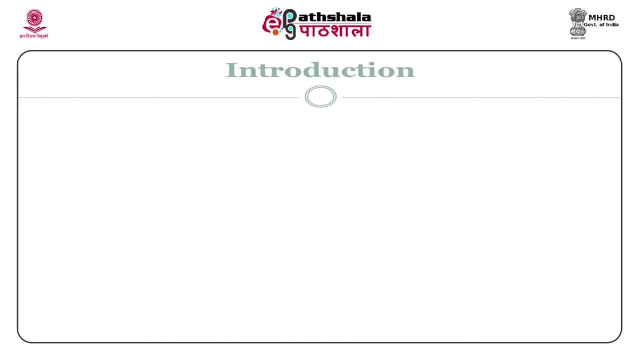 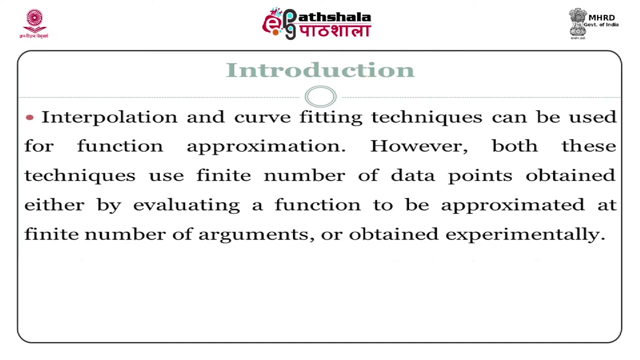 this function by a polynomial function, p. This is because computational capabilities of digital computers are restricted to arithmetic operations and evaluation of a polynomial function involves only basic arithmetic operations. Interpolation and curve fitting techniques can be used for function approximation. However, both these techniques use finite number of. 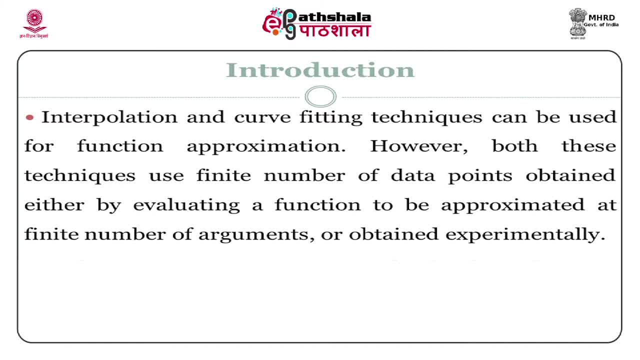 data points obtained either by evaluating a function to be approximated or by evaluating a function to be approximated. The function is either approximated at finite number of arguments or obtained experimentally. Such approximations are completely dependent on these finite data values and do not use 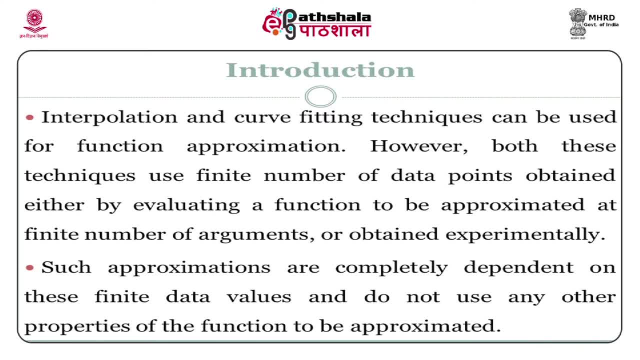 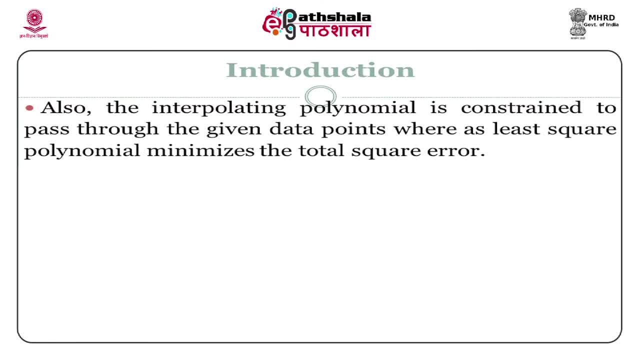 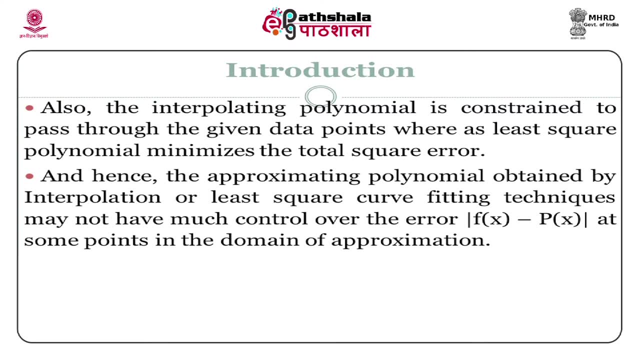 any other properties of the function to be approximated. Also, the interpolating polynomial is considered to pass through the given data points where as least square polynomial minimizes the total square error and hence the approximating polynomial. 唉, dooой m campaigns are considered to be mod-ererolla term decolonize and. 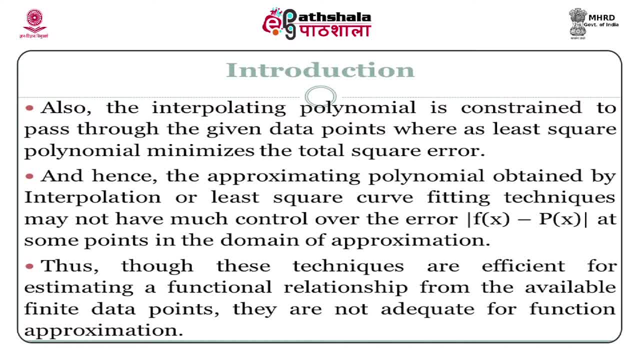 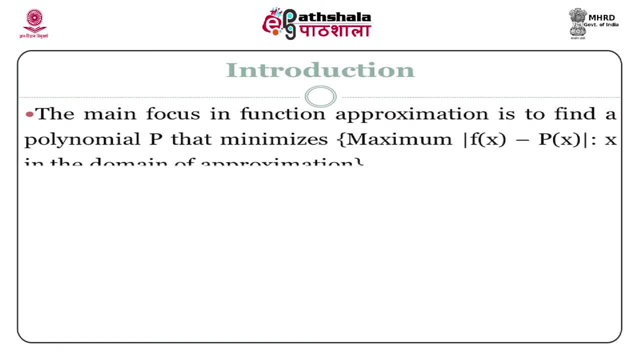 interpret the co-efficient aspects: 、 combat mating sogenan acne function. proyecto is designed for uh polymer aviation function or function approximation that minimizes the maximum of individual error. that is mod fx minus px and x in the domain of approximation. So we try to compute error at each point in the domain of approximation and we try. 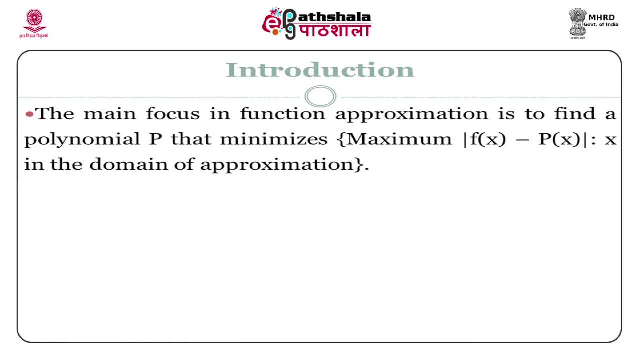 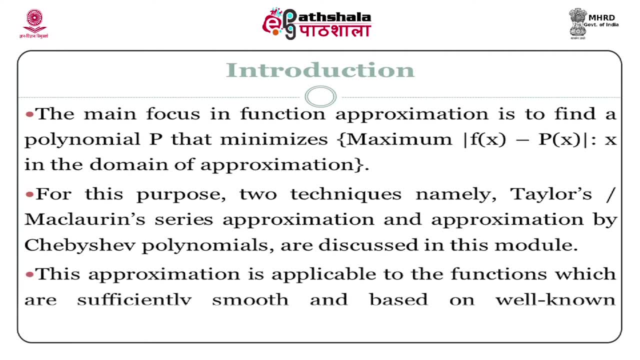 to maximize that. and then we want to find out a p which will minimize this maximum error. For this purpose two techniques, namely Taylor's or Maclaunay series, approximation and approximation by Chebyshev polynomials are discussed in this particular module. For Taylor's polynomial approximation, the main tool is the Taylor's theorem, which 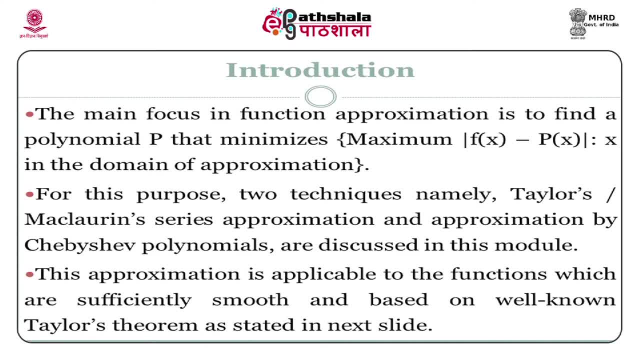 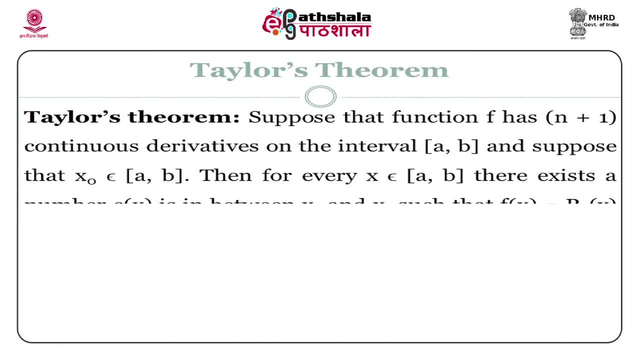 is the Venlun theorem in calculus which says, or which states as follows: Suppose that function f has n plus 1 continuous derivatives on the interval a, comma, b and suppose that x0 belongs to ab, then for every x belonging to interval ab, there exists a. 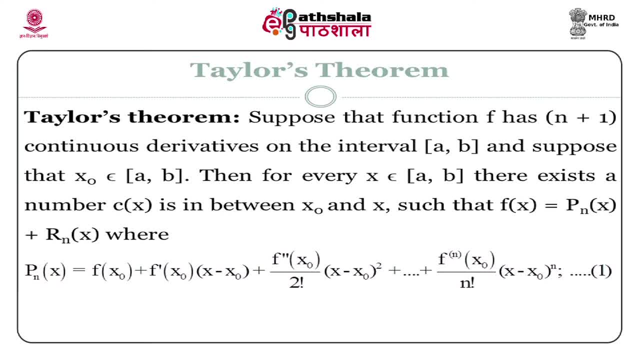 number cx n between x0 and x, such that fx is equal to capital plus x. So fx is equal to capital plus x. So fx is equal to capital plus x. So fn plus pnx plus rnx, where capital pnx is given by fx0 plus f, dash x0 into x minus. 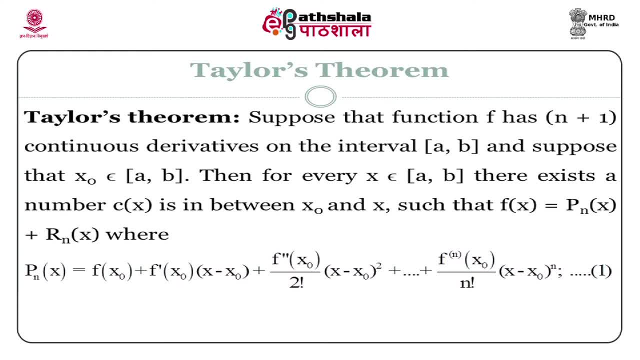 x0 plus f, double dash: x0 upon 2 factorial into x minus x0, whole square plus fnx0 upon n factorial into x minus x0, raise to n. So we are taking sum up to this nth term, So this becomes a nth degree polynomial function. 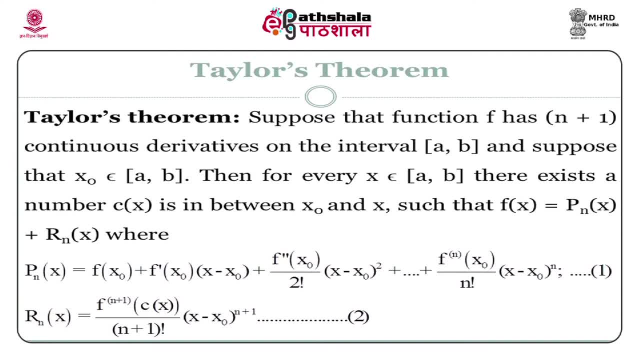 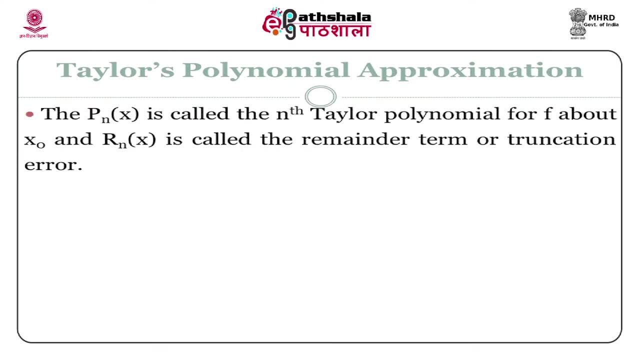 And rnx is given by fn plus 1 at cx. So nth plus 1th derivative at Cx divided by n plus 1, factorial into x minus x0 raised to n plus 1.. The capital, Pnx, is called the nth Taylor's polynomial for f about x0, and Rnx is called 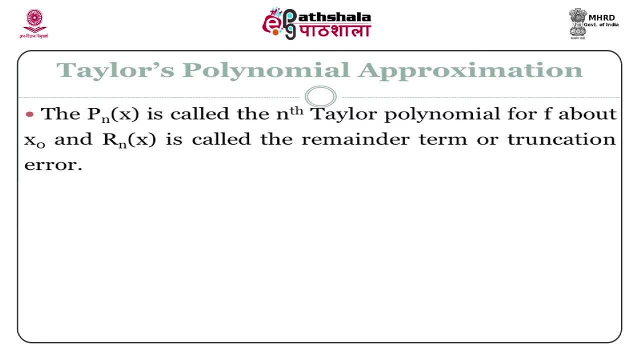 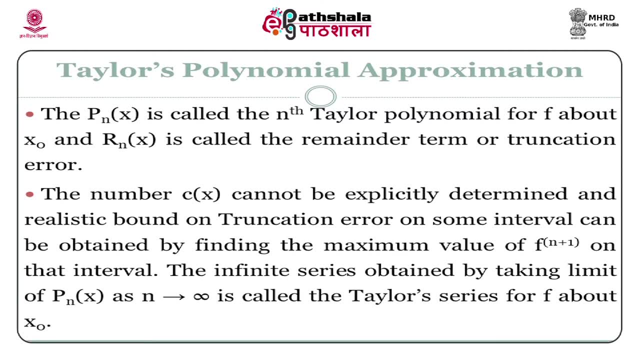 the remainder term or the truncation error. The number Cx cannot be explicitly determined and realistic, bound on truncation error on some interval, can be obtained by finding the maximum value of fn plus 1 on that interval. The infinite series obtained by taking limit of capital Pnx as n tend to infinity, is called: 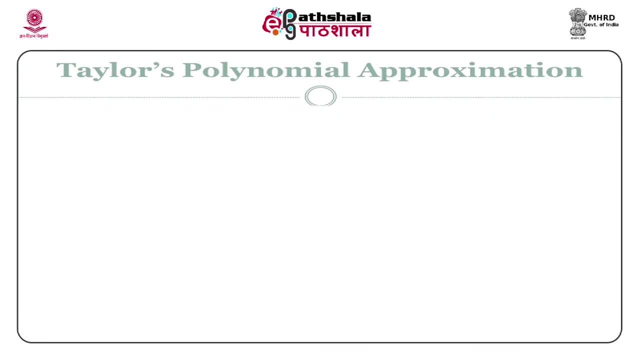 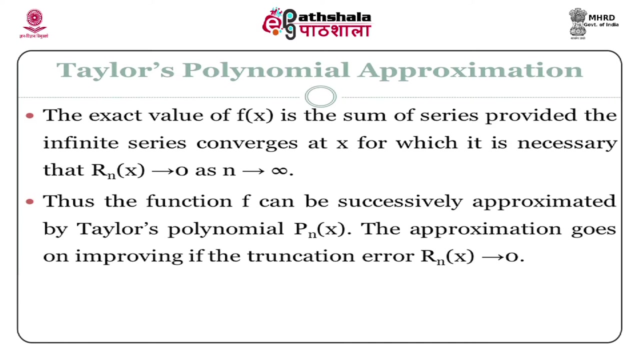 the Taylor series for f about x0.. The exact values of fx is the sum of the series provided. the infinite series converges at x, for which it is necessary that Rnx tends to 0.. Thus the function f can be successively approximated by Taylor's polynomial Pnx. 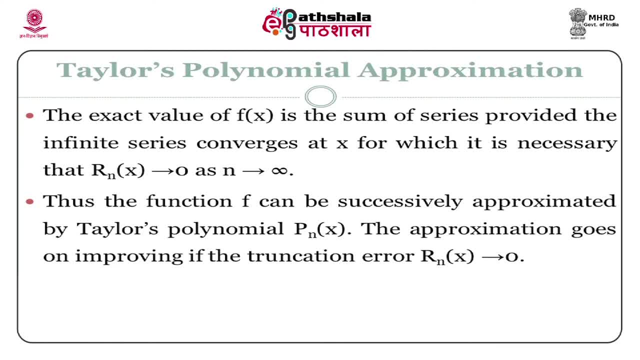 The approximation goes on improving if the truncation error Rnx tends to 0.. If x0 is equal to 0, then the Taylor's polynomial or series, or are called, actually is oblique, are called Maclaurin's polynomial or series. 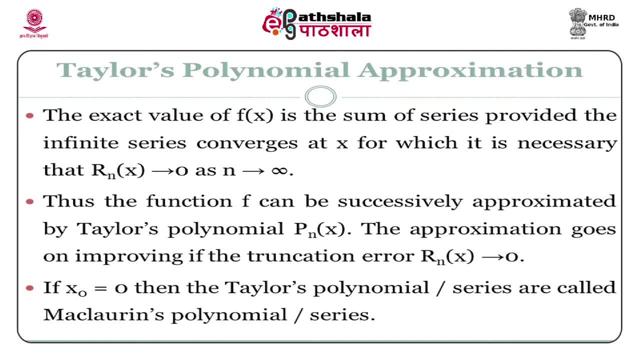 So Taylor's polynomial at x0, equal to 0, is 0.. Thank you. This Maclaurin's polynomial at x0 at 0 is Maclaurin's polynomial for f, and same is the case for the series. These Maclaurin's polynomials are given as under: 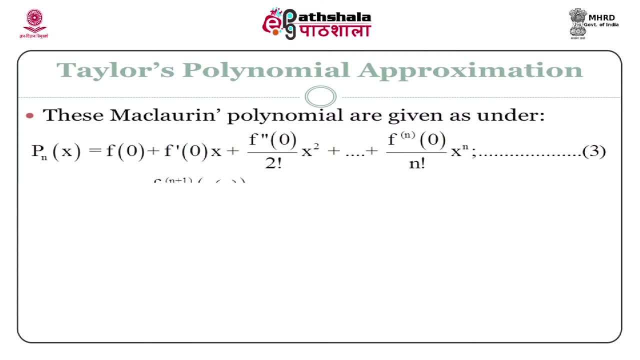 So Pnx will be f0 plus f dash 0 into x plus f double dash, 0 upon 2 factorial into x square and go on summing up to this up to nth term, that is fn0 upon n factorial into x. raise to n. 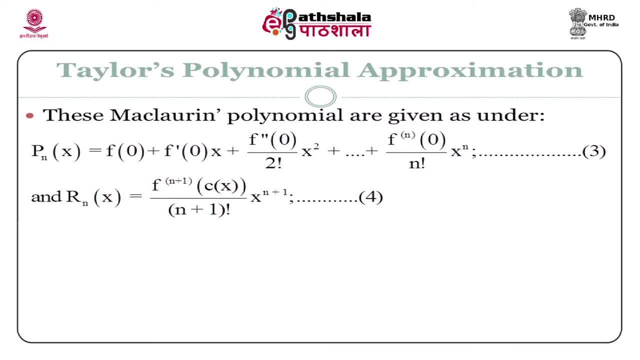 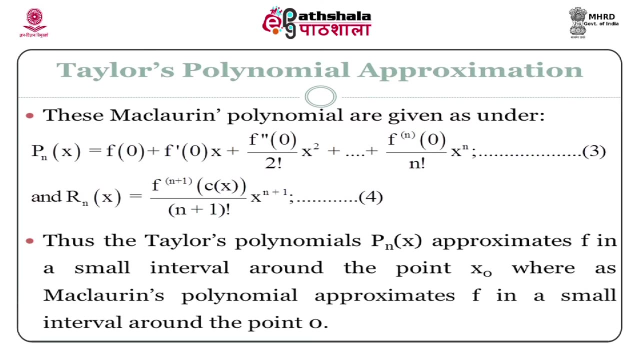 And Rnx in that case will be fn plus 1 at Cx. upon n plus 1, factorial x raise to n plus 1 and Cx will be some point in the interval 0 and x. Thus the Taylor's polynomial Pnx approximates f in a small interval around the point x0,. 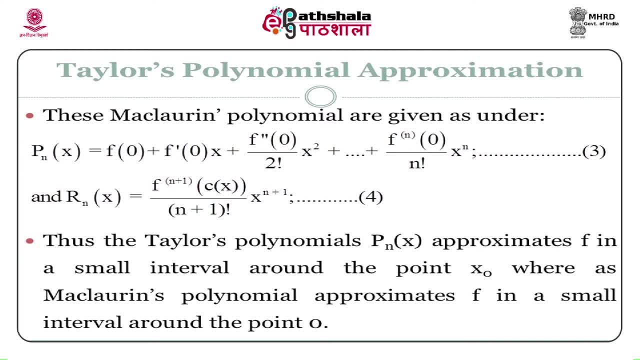 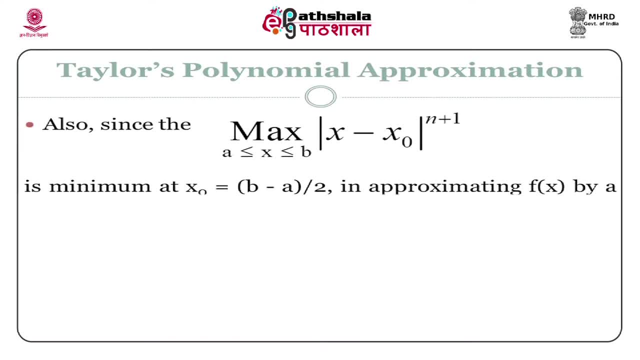 whereas Maclaurin's polynomial approximates f in a small interval around the point 0.. Also, since the x minus x0 is minimum at x0, equal to b minus a by 2 and maximum value x minus x0 over the interval this ab. 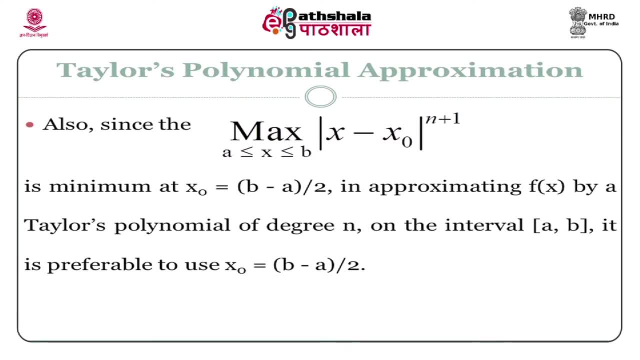 Thank you, will be minimum at b minus if x 0 is equal to b minus a by 2. in approximating f- x by Taylor's polynomial of degree n on the interval a- b, it is preferable to use x 0 as b minus. 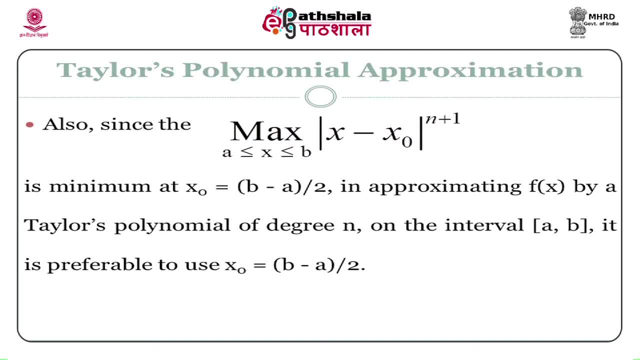 a by 2.. So what we are saying here is that if x 0 is not given to you in advance and if you want to approximate a by polynomial on the interval a- b, then we can choose x 0 as b minus a by 2, as that will give me the least value of the maximum of mod x minus. 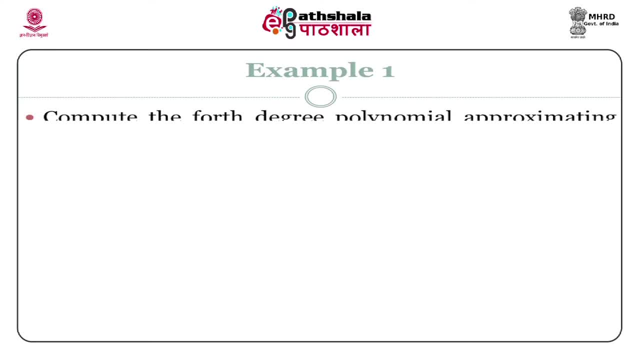 x 0. Now we take example 1.. For example, let us take compute the fourth degree polynomial approximation to the function f: x equal to e raised to cos x, 1 for x belonging to minus 0.5 to 0.5 and 2 for x belonging to pi by 4 comma, 3 pi by 4.. Since the interval is around, 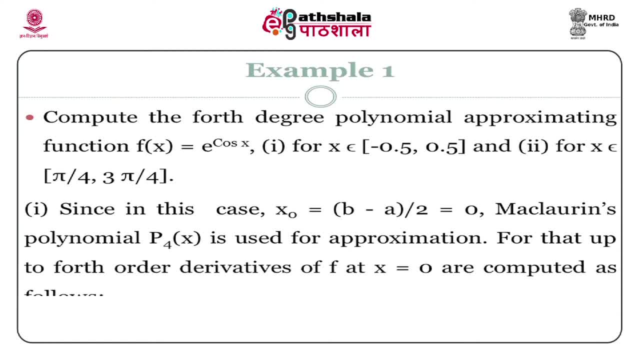 x 0 equal to 0, first interval is around x- 0 equal to 0.. Maclaurin's polynomial p 4- x is used for approximation For that. up to fourth order derivatives of f at x equal to 0 are computed as follows: f- 0 equal to 2.7183, f- dash x. 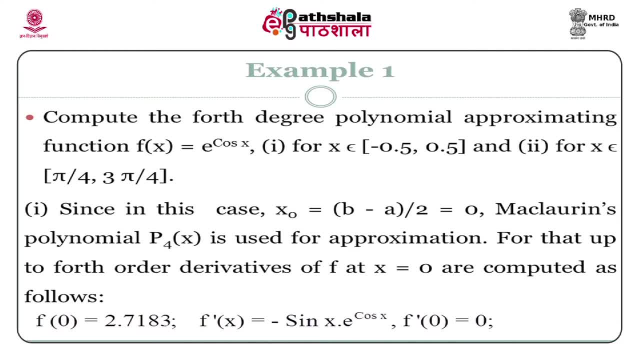 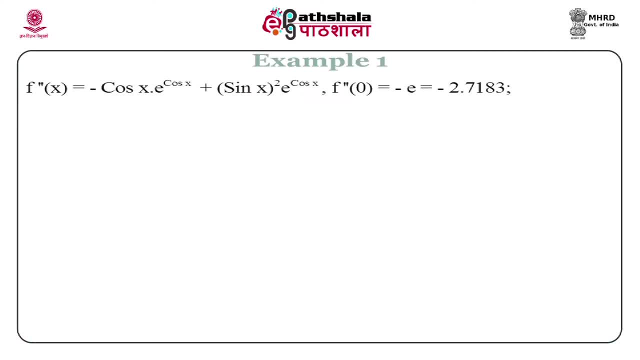 equal to minus sin x into e raised to cos x into e raised to cos x comma, f dash 0 and therefore f dash 0 is equal to 0.. Then f double dash x equal to minus cos x into e raised to cos x plus sin x whole square into e raised to cos x. 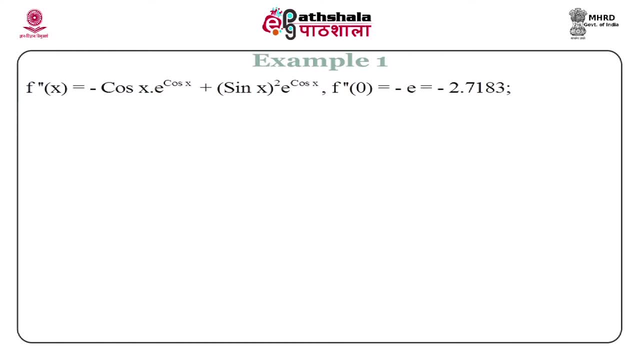 Therefore, f double dash 0 is equal to minus e, that is, minus 2.7183,. f triple dash x is equal to sin x into e raised to cos x, plus 1.5 into sin 2 x into e raised to cos x minus. 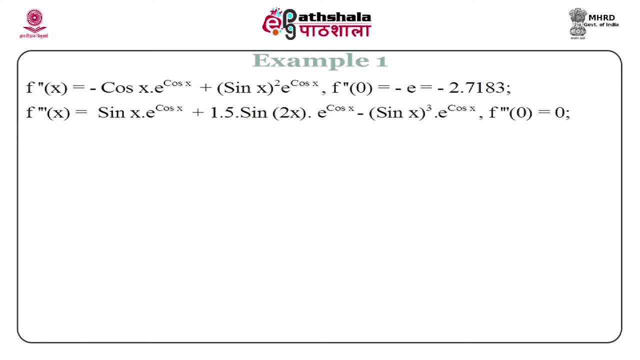 sin x cube into e raised to cos x. Therefore f triple dash 0 will be 0 and similarly f 4 x will be cos x into e raised to cos x minus sin whole square into e raised to cos x plus 3 cos 2 x into e raised to cos x. 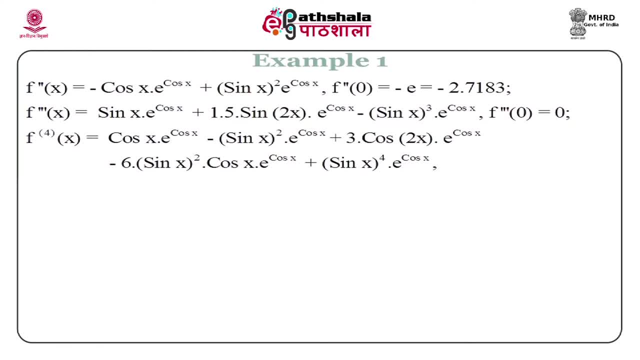 into cos x, e raise to cos x plus sin raise to 4, e raise to cos x and therefore F 4: 0 will be equal to 4 into e, that is, 10.8732.. These derivatives are used using elementary calculus. Putting these values in 3, we get the desired. 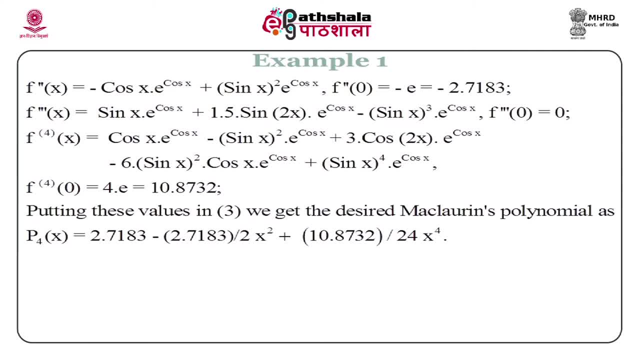 Maclaurin's polynomial as P 4 x is equal to 2.7183 minus 2.7183 by 2 into x square, plus 10.8732 by 24 into x raise to 4.. The 2 terms are not there: x and power, x cube. 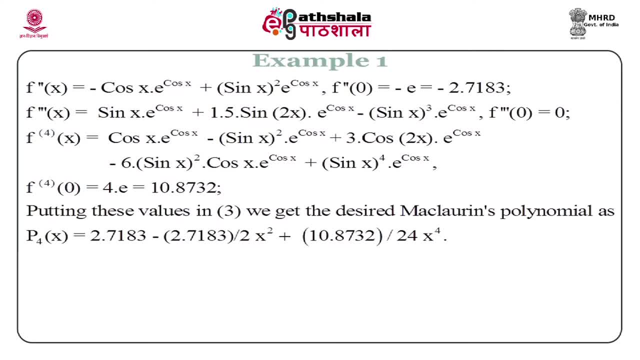 terms are not there because F dash is 0 and F triple dash is 0.. The values of this polynomial at some point x equal to 0.12, we can compute by using this polynomial and that gives us the following: me the value as 2.698.. We get estimated value at x equal to 0.12 as 2.716437, and since f 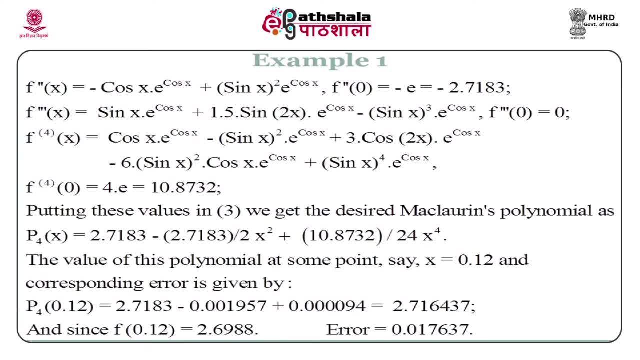 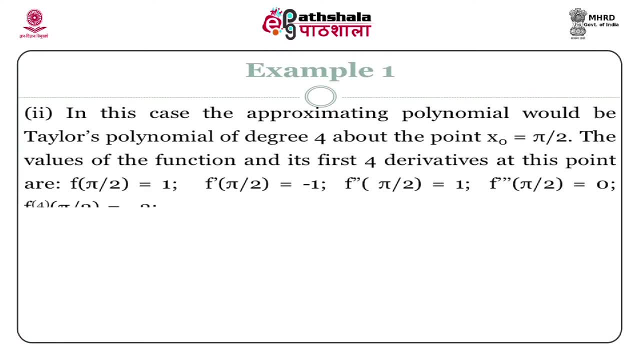 exact value of f at 0.12 is 2.698. at error is equal to 0.17637.. Second part of this example: in this case the approximating polynomial would be a Taylor's polynomial of degree 4 around the point x0, equal to pi by 2.. As your interval is pi by, 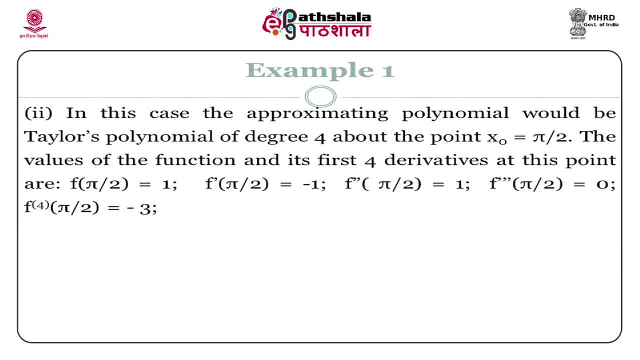 4 to 3, pi by 4, its midpoint is pi by 2.. The values of the function and its first four derivatives. at this point, first four derivatives. forms are already computed earlier. the same thing we are using Now. instead of putting x equal to 0 there, we are putting now x equal. 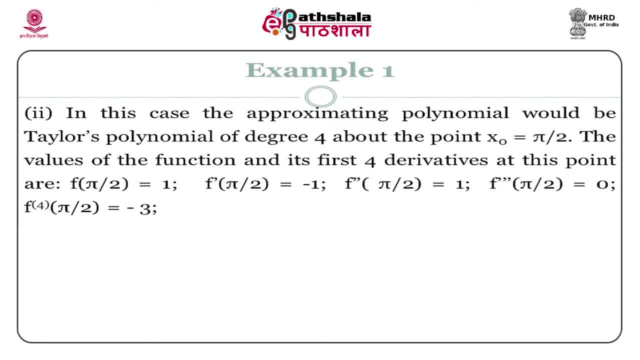 to pi by 2 and we will get f pi by 2 equal to 1, f dash pi by 2 equal to minus 1, f double dash pi by 2 will be equal to 1 and f triple dash pi by 2 will be equal to 0 and f 4 pi. 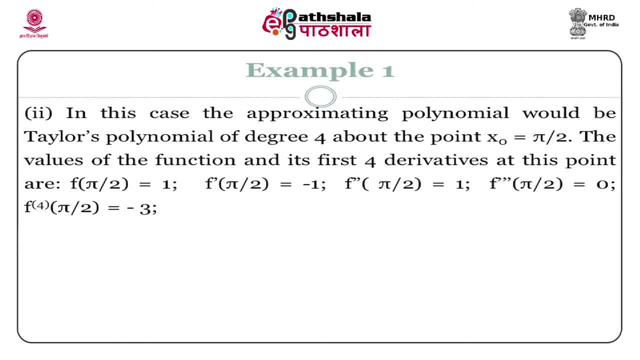 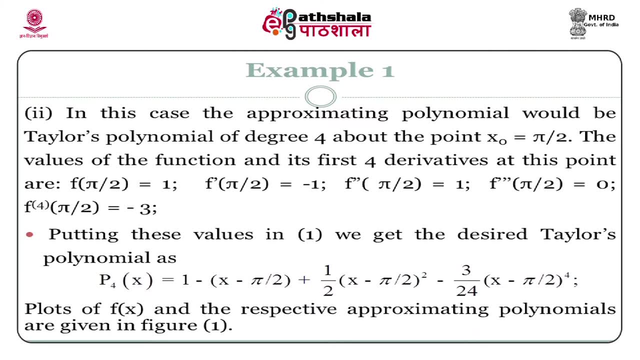 by 2 will be equal to minus 3.. You can compute that easily from the formula given for these derivatives In the part 1,. so putting these values in 1,, we get the desired Taylor's polynomial as p4 x equal to this. The plots of this exact function and the polynomial approximation: 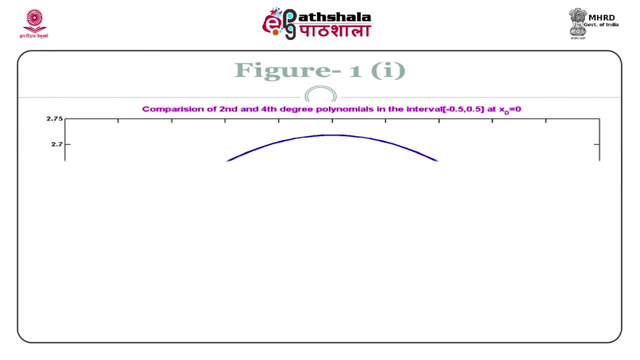 are given in figure 1 and 2.. The first figure gives me the approximation over the interval 0.5 to minus, 0.5 to 0.5, and the red line gives me the second degree polynomial approximation and blue line gives me fourth degree polynomial approximation. So you take first two terms. 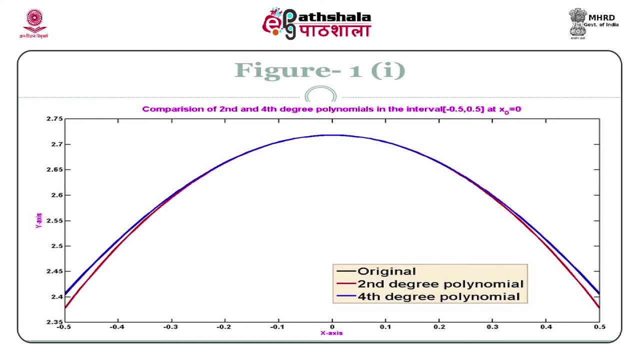 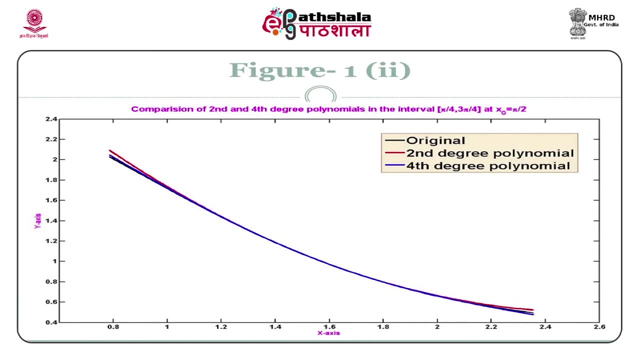 is second degree polynomial approximation. four terms will give me fourth degree polynomial approximation to the original function. You can see that original function almost matches the fourth-degree polynomial approximation function And if you take the second part of the first example and the second-degree polynomial, if you take you can see that second degree polynomial it will mismatch. 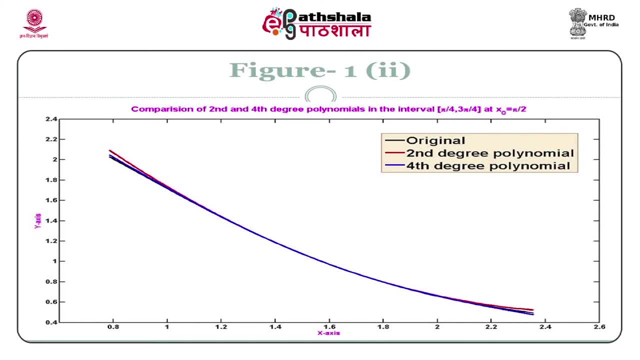 it there towards the end. Otherwise, fourth-degree polynomial and the original function both match well If the function f is infinitely differentiable and if nth derivative of f has is zero to half number of endings plus 1 and minus 1.. I am able to compute Н you. 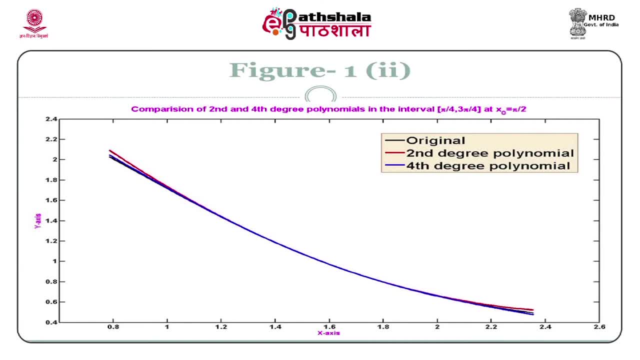 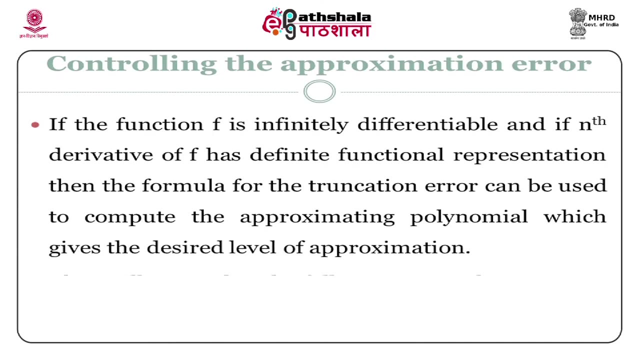 definite functional representation, then the formula for truncation error can be used to compute the approximating polynomial which gives the desired level of approximation. This is illustrated in the following example. So what we are saying is that if the function f is infinitely differentiable, you can take polynomial up to any degree to approximate. 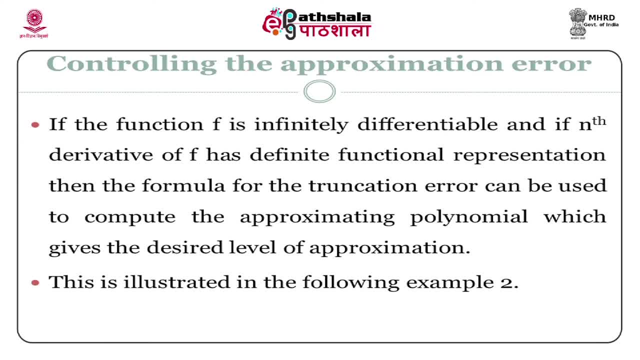 the function f And as the degree of the polynomial increases, the approximation goes on improving if the Taylor series converges And therefore we can use this to get the desired level of approximation. So, for example, if you take f x equal to cos 2, x over the integral minus, 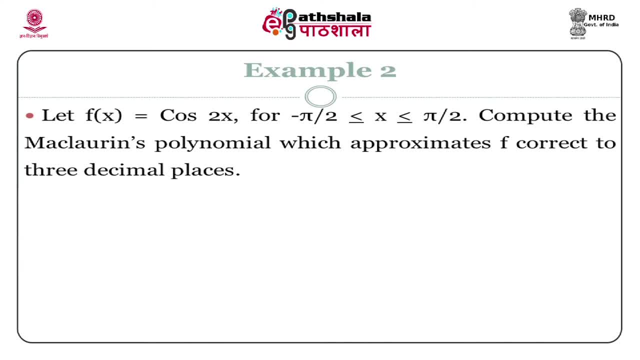 pi by 2, less than or equal to x less than or equal to pi by 2, compute the Maclaurin's polynomial which approximates f correct to three decimal places. So since nth derivative of f, in this case, is given by f n x equal to 2, raised to n into: 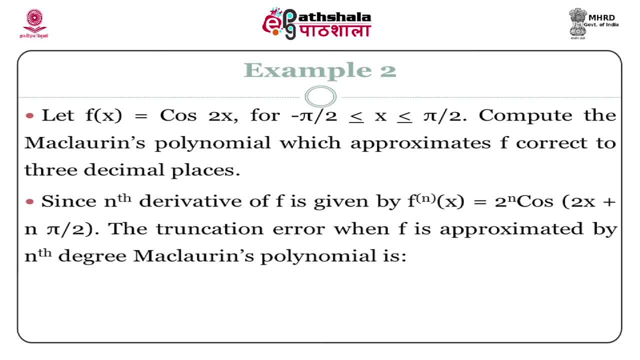 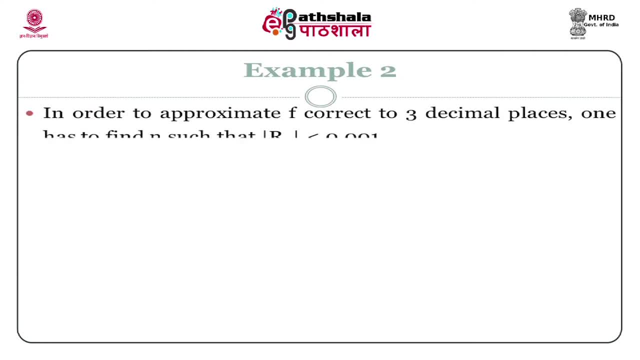 error. So this is the truncation error. So this is the truncation error. So this is pi by 2 to pi by 2.. In order to approximate f correct to three decimal places, one has to find n such that mod rn is less than or equal to 0.001.. This yields n equal to 12.. 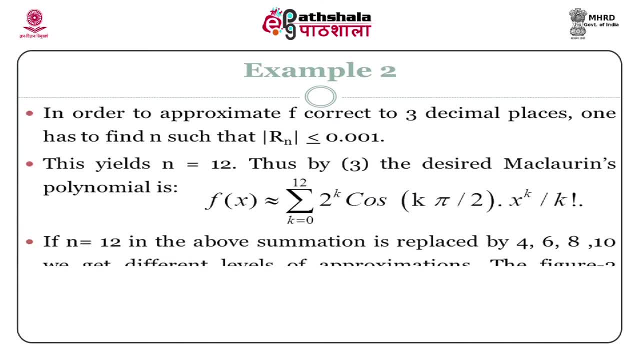 We can compute that and you can see that n will be equal to 12.. Thus by 3, that means the formula 3, desired Maclaurin series, polynomial approximation is given by: fx is equal to k, equal to 0 to 12.. This is 2. raise to k into cos, that is fkx, the kth derivative of f. 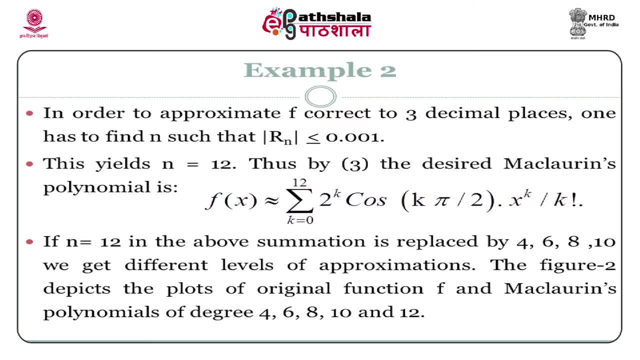 into x, raise to k upon k, factorial. So this is what we are saying, that this is the 12 degree polynomial. If you truncate this to 10, you will get 10 degree polynomial. If you truncate it to 8, you will get 8 degree polynomial approximation, 6 degree. Like that you can always get various. 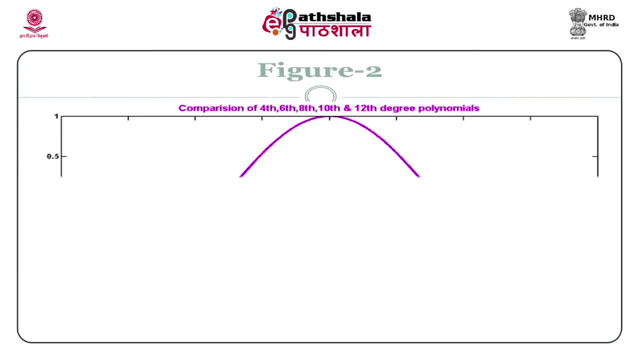 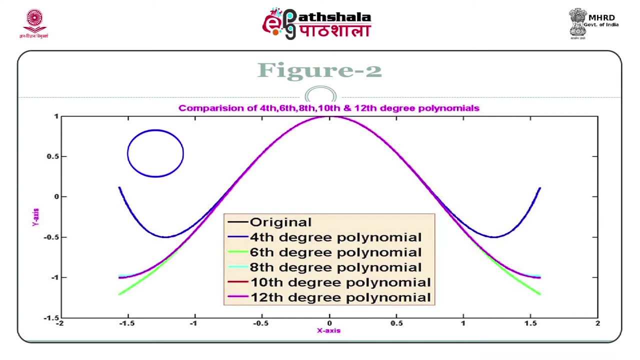 degrees of polynomial approximations. here This figure 2 gives me the various polynomial approximations to the function. One is the blue line gives me the fourth degree polynomial approximation to the original function. Original function is of course represented by black. Then green gives me the sixth degree polynomial approximation. Eighth degree polynomial approximation. 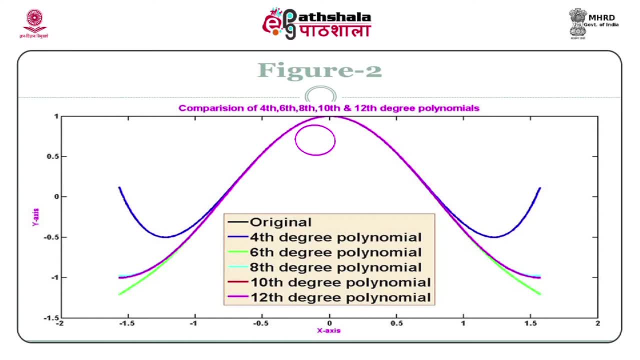 polynomial is given in blue, Tenth degree is given in red and twelfth degree given in magenta. So we can get various polynomial approximations to the function f. Observe that fourth degree and sixth degree polynomial approximation do not match so well. 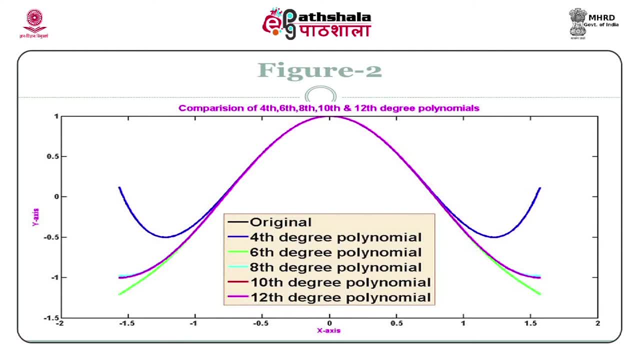 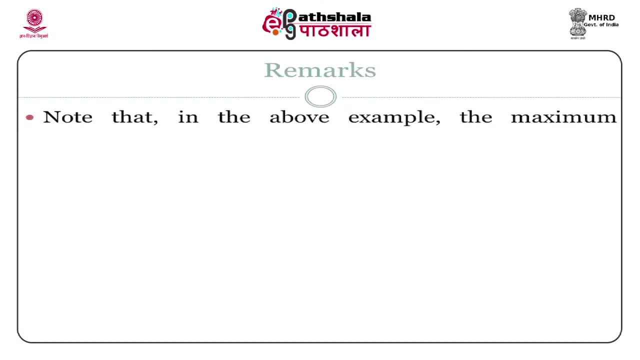 but eighth degree is relatively okay. but tenth and twelfth degree match very well and they are in fact almost coincident on that. Note that in the above example the maximum possible truncation error over the entire interval of approximation has been controlled And therefore the values of value of n, the 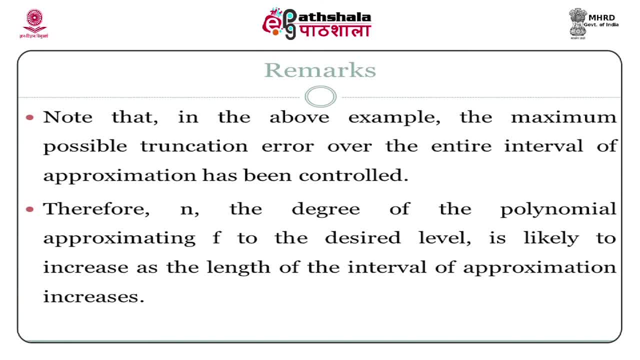 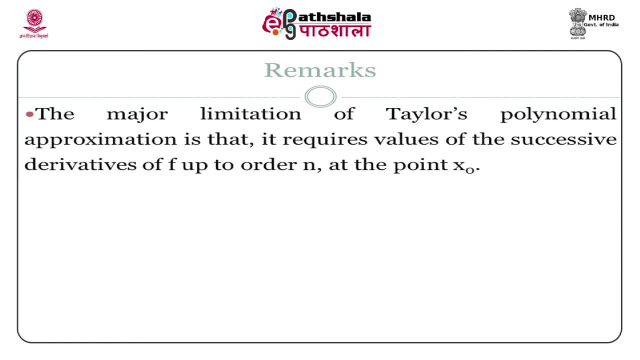 degree of the polynomial approximating f to the desired level is likely to increase as the length of the interval of approximation increases. The major limitation of Taylor's polynomial approximation is that it requires the values of f, values of the successive derivatives of f, up to order n at the point x, 0.. Hence, 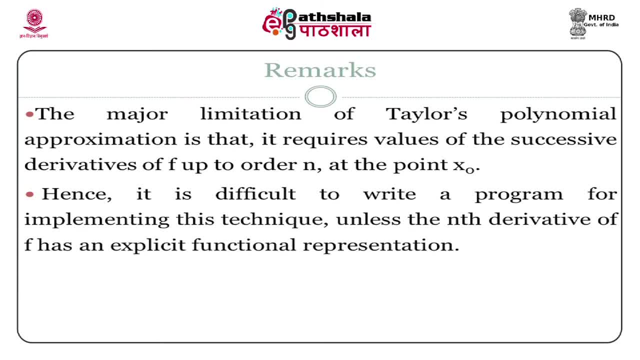 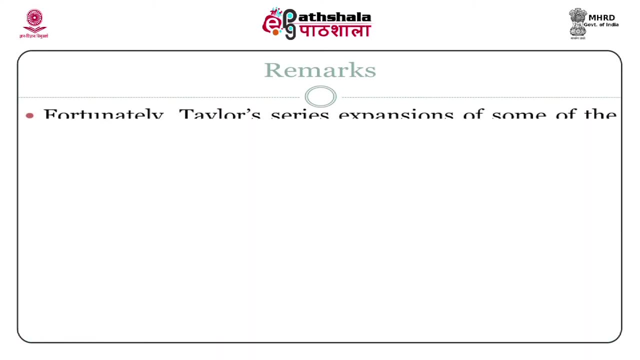 it is difficult to write a program for implementing this technique unless the nth derivative of f has an explicit functional representation. Time complexity of such a program will significantly depend on how complex are the functional forms of f and its nth derivatives are, Fortunately, Taylor series expansions of some of the standard functions like sin x, cos. 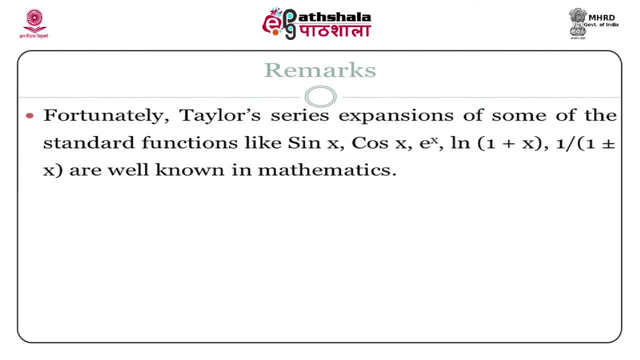 x e raise to x, ln. 1 plus x, 1 upon 1 plus x, plus or minus x, you can say as well. as are well known in the mathematical world. So we can write a program for implementing this technique. 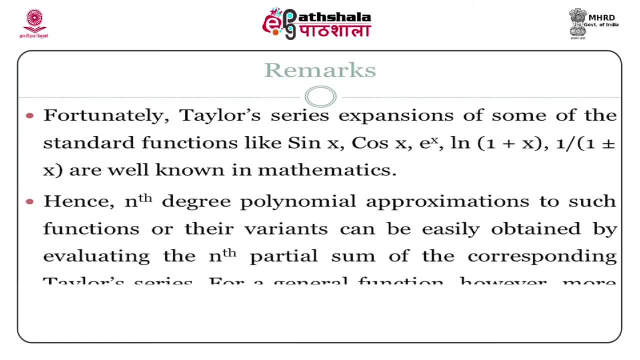 In mathematics. hence, nth degree polynomial approximation to such functions or their variants can be easily obtained by evaluating the nth partial sum of the corresponding Taylor series. For a general function, however, more sophisticated techniques are required. So approximation by Chebyshev polynomials, the Taylor's polynomial approximation, can be viewed as approximation. 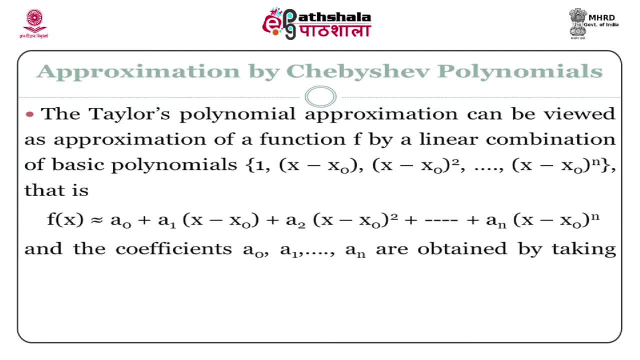 of a function f by a linear combination of the basic polynomials 1, x minus x 0, x minus x 0 square, x minus x 0. raise to n. That is, f is equal to a zero plus a1. into x minus x0a2, into x minus x0, square like. 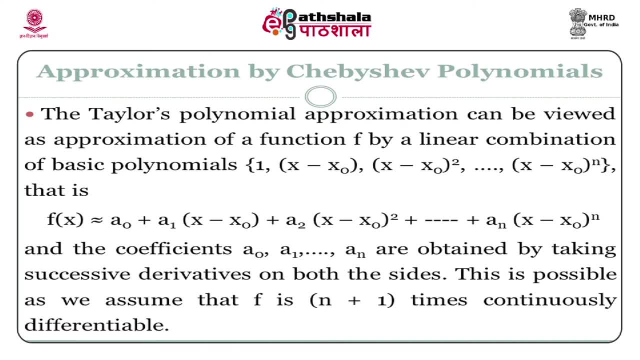 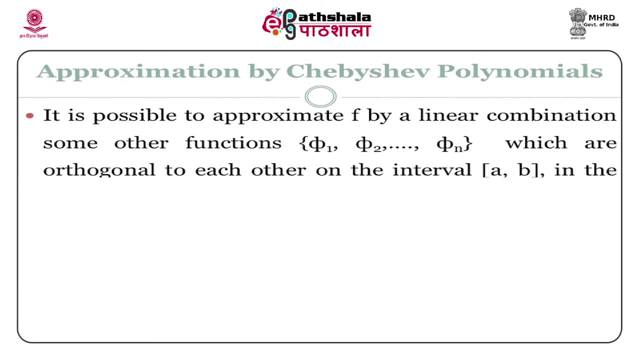 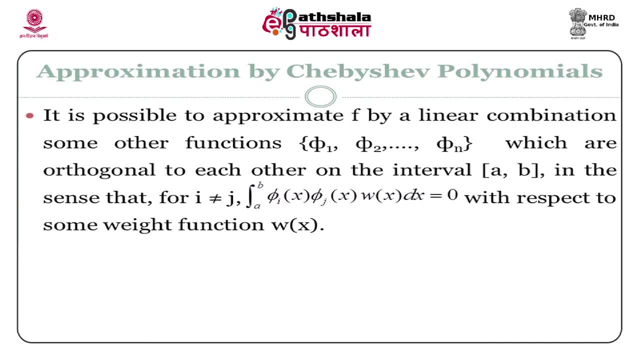 which are orthogonal to each other on the interval a- b, in the sense that for i not equal to j a to b, phi i x into phi j x, w x, d x is equal to 0 with respect to some weight function, w x. Thus f x is given by a 1, phi 1 x plus a 2, phi 2 x plus a n, phi n x and. 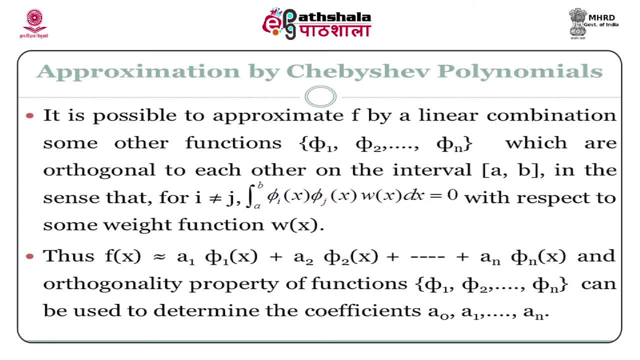 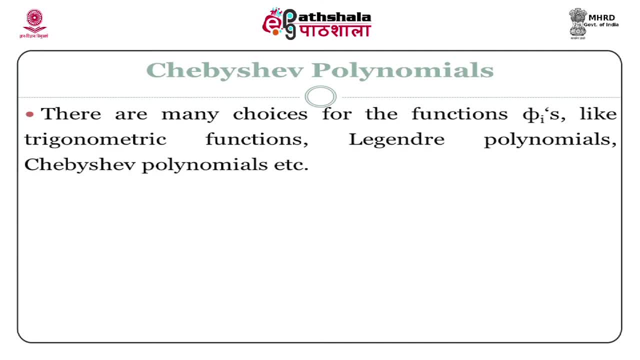 the orthogonality property of the functions phi 1, phi 2, phi 3, phi n can be used to determine the coefficients a, 0, a, 1, a, 2, a, 3, a n. There are many choices for the functions phi i's. 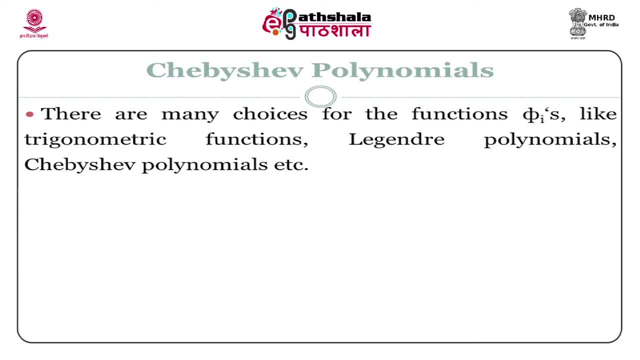 like trigonometric functions. we can use Legendre polynomials, we can use Chebyshev polynomials, we can use etcetera and many more Bessel's functions we can use. for example, In this module the Chebyshev polynomials are used to approximate f, as these polynomials 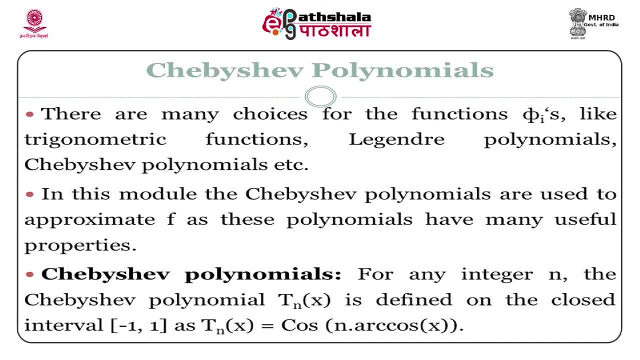 have many useful properties. Chebyshev polynomials. so first we will understand what are Chebyshev polynomials. For any integer n, the Chebyshev polynomial Tn x. Tn x is defined on the closed interval minus 1 to 1 as Tn x, equal to cos of n, into r cos. 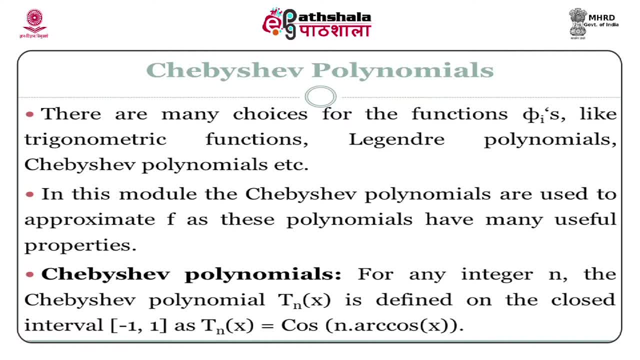 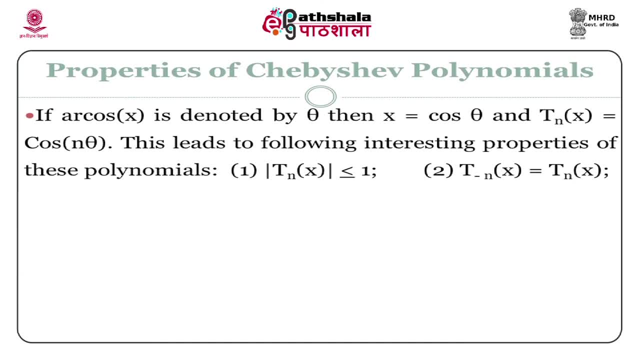 x, that is, cos inverse n into cos inverse x, So cos of n into cos inverse x. If r cos x is denoted by theta, then x equal to cos theta and Tn x equal to cos n theta. This leads to the following interesting properties of these polynomials: Mod Tn x is less than. 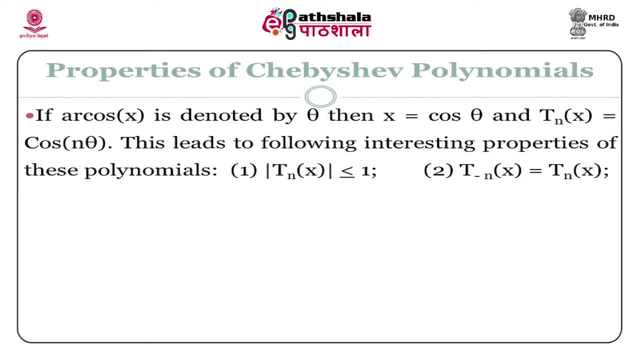 1,. that is why, quite clear: T minus n x is equal to Tn x, As cosine of minus n theta will be same as cos n theta. Now, if you take T0 x, so what will be T0 x? So in that case we will be getting here r cos x as pi by 2, n pi by 2. 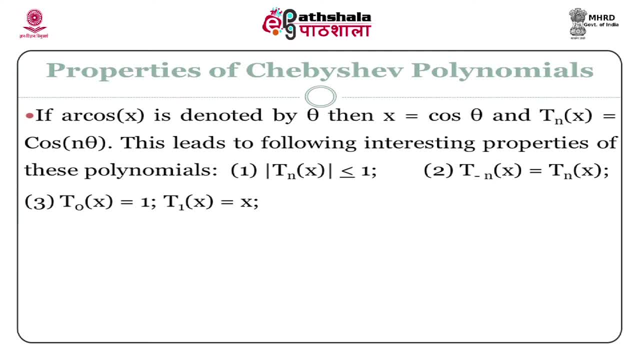 and therefore cos n pi by 2 will be equal to. we will get T0 x will be equal to 1.. T1 x will be equal to x, and Tn plus m x plus Tn minus m x will be equal to what. So that? 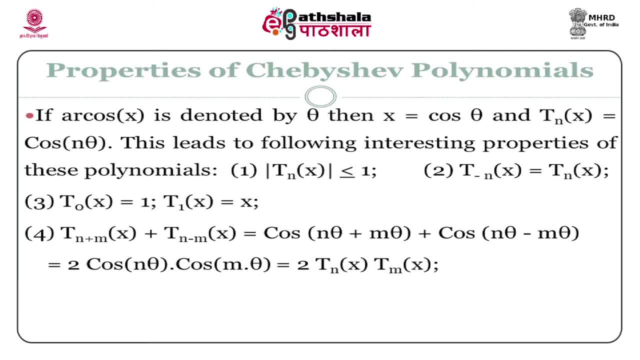 will be equal to cos n theta plus m theta plus cos n theta minus m theta, and when you add the two will be 2 cos n theta into cos m theta. but cos n theta is Tn x and cos m theta is Tm x and therefore that will be less. So when you are writing here T0 x, we are taking. 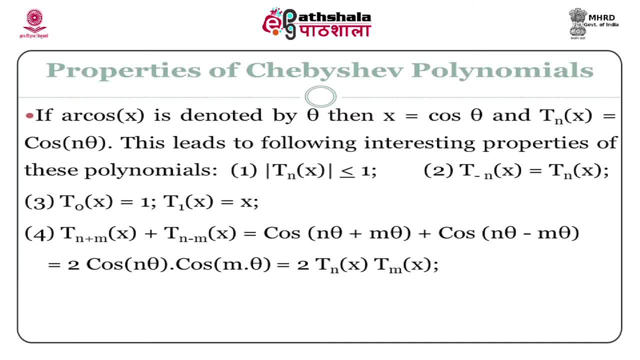 n equal to 0. Therefore, cos 0 is 1.. And when you are taking n equal to 1, I will get T1, x, that is cos 1. x is equal to x. Fifth property says that. this fourth property. 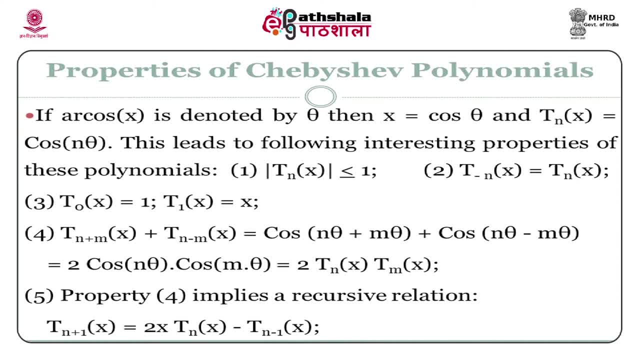 implies the recursive relationship, if I take m equal to 1.. So then in that case, Tn plus 1 plus Tn minus 1, x is of course minus m by 2.. So then, cos m theta and cos m theta. will be 2 cos n theta into cos m theta, but cos m z equal to 1.. For the first propertides, cos m theta will do the same thing that we have just done, And in that case the factor of n. 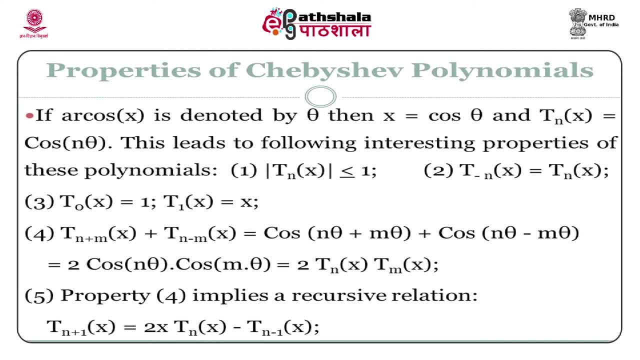 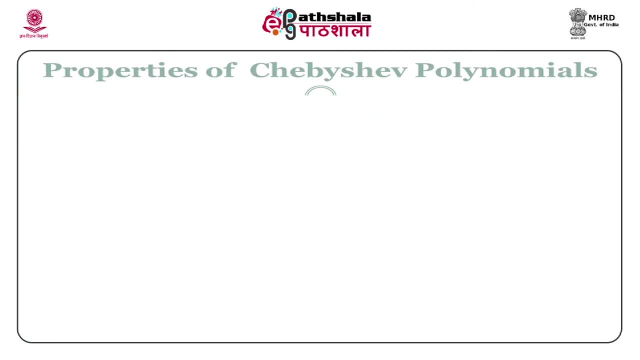 minus 1 will be equal to 2 Tn into T1 x, but T1 x is x and therefore I can say that Tn plus 1 x equal to 2 x into Tn x minus Tn minus 1 x. 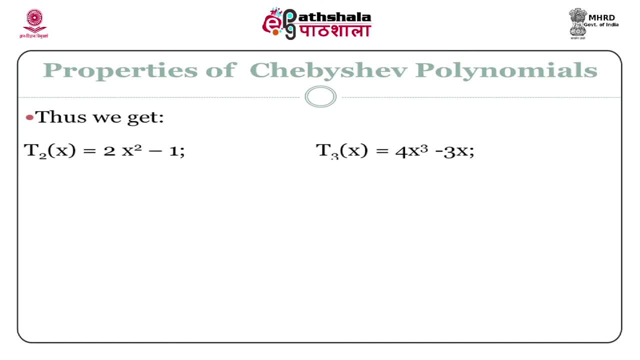 Thus we get T2 x equal to 2 x square minus 1 using this recursive relationship: T3 x equal to 4 x cube minus 3 x. T4 x equal to 8 x raise to 4 minus 8 x square plus 1, T5. 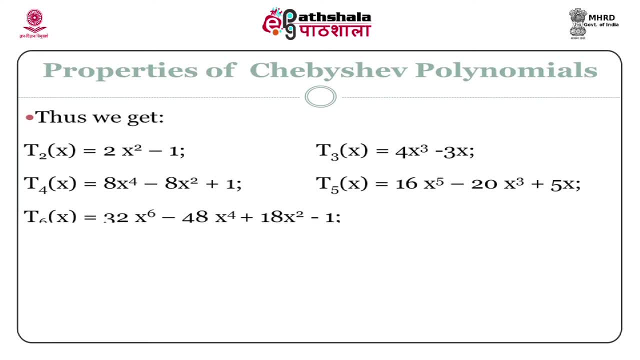 x will be 16 x raise to 5 minus 20 x cube plus 5 x and T6 x will be equal to 32 x raise to 6 minus 48 x raise to 4 plus 18 x square minus 1.. 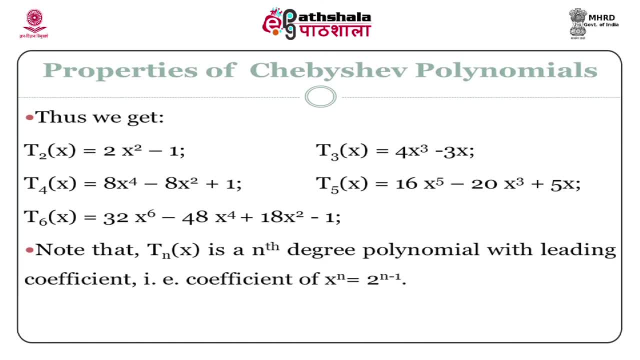 Note that Tn is a nth degree polynomial with leading coefficient, that is, coefficient of x. raise to n. equal to 2, raise to n minus 1.. The graph of these functions is given in the following figure 3.. We can see that these are the graphs of various functions. 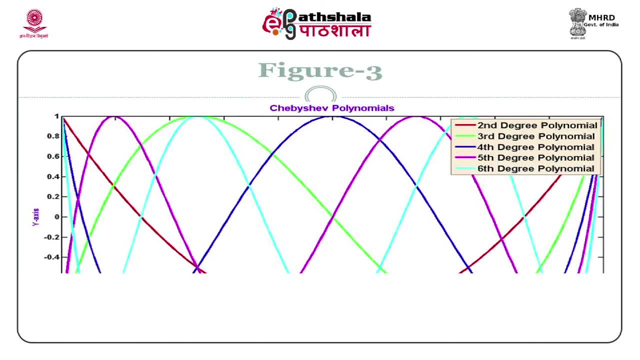 So second degree polynomial function, The first degree say zero, at degree T0 is 1, so constant T1 is x, so that is straight line. second: t2x onwards up to t6x are given in this figure and various colours distinguish. 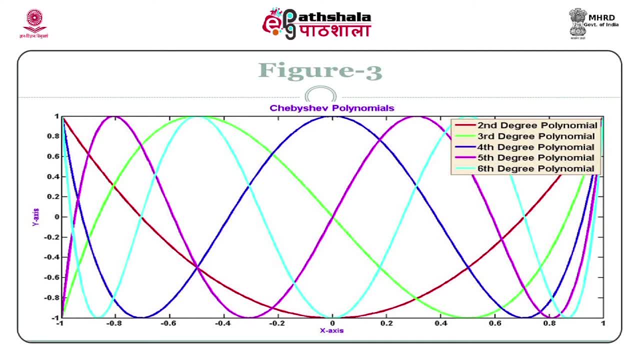 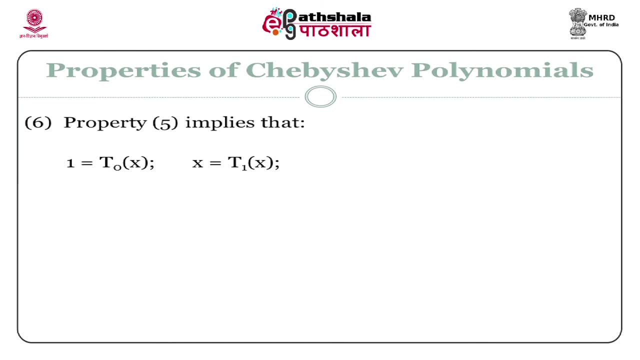 between these functions. Now, if you do the reverse exercise, that means from the equations which are given in property 5, we are getting tnx in terms of powers of x. Now we will get powers of x in terms of tnx by combining those equations in property 5.. So 1 is equal to t0x, x equal to t1x. 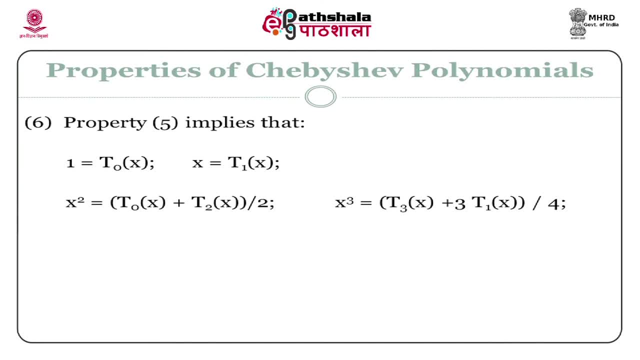 x square will be equal to t0x plus t2x by 2, x cube x will be equal to t3x plus 3 times t1x by 4, x raised to 4 will be equal to t4x plus 4, t2x plus 3, t0x by 8, and so on. So. 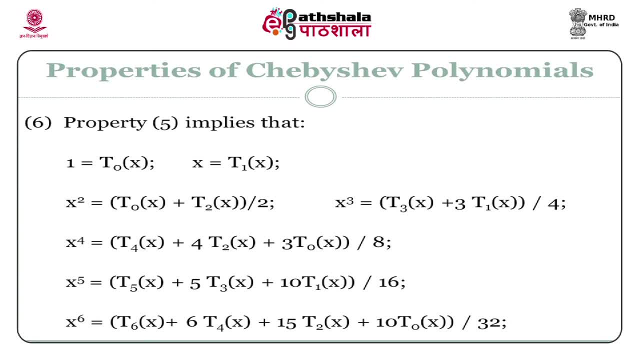 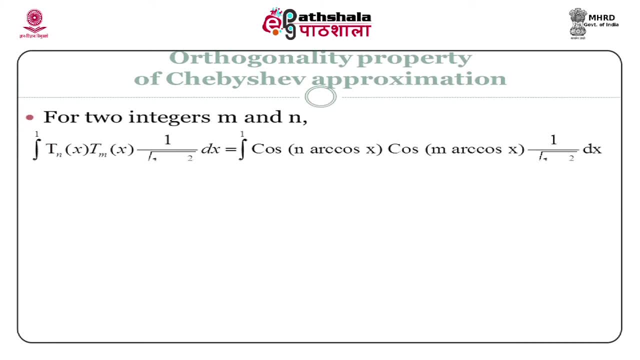 all these properties you can. the simple manipulation will give you these properties. So for orthogonality property, we are talking about Chebyshev, polynomial for two integers, m and n, minus 1 to n, tnx into tmx, into 1, upon under root of 1 minus x square dx. this: 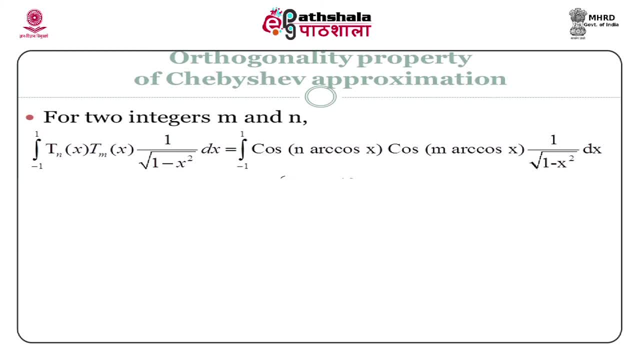 is equal to t, So that will be equal to t2x by 3 root of t3x plus t1x by 2, t2x divided equal to minus 1 to 1. cos n r, cos x into cos m r, cos x into 1 upon n root of 1 minus x. 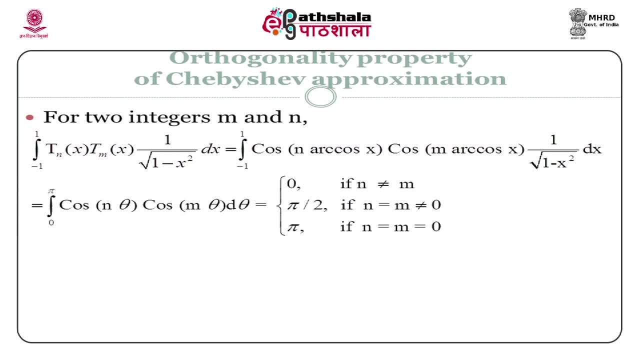 square dx. Now if I put r cos x equal to theta in this integral, then you will get 1 upon n root of 1 minus x square minus 1 upon n root of 1 minus square dx equal to d theta and the whole thing will be converted to 0 to pi cos. 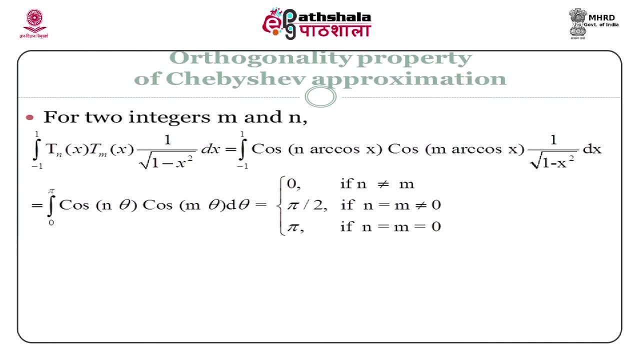 n theta cos m theta d theta. And it is well known that this interval will be equal to 0 if n is not equal to m, and pi by 2 if n is equal to m but they are not equal to 0. and it will be equal to pi if n is equal to m and both of them are 0. Thus the Chebyshev. 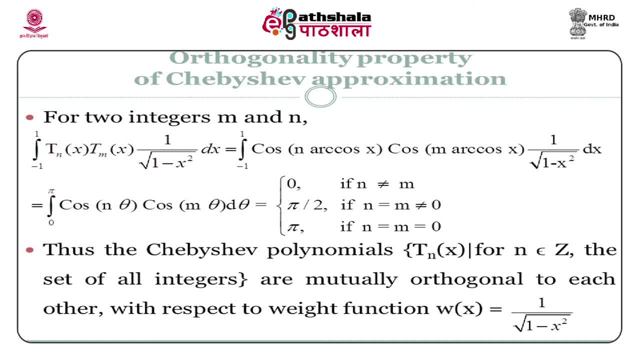 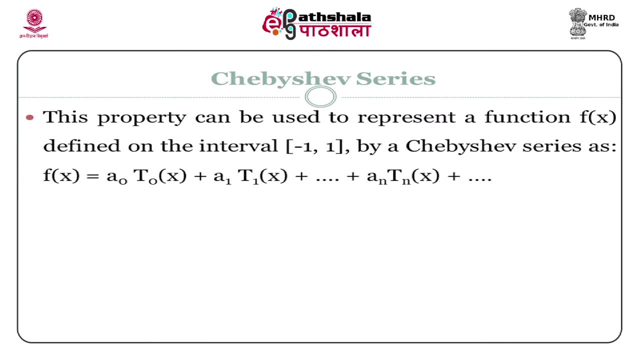 polynomial t, n, x for n belonging to z. the set of all integers are mutually orthogonal to each other with respect to weight. function w x equal to 1 upon n root of 1 minus x square. This property can be used to represent a function f x defined on the interval minus 1 to 1 by: 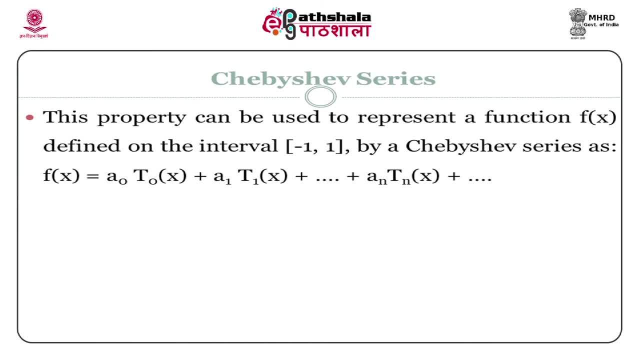 Chebyshev series like this: a 0 t 0 x plus a 1 t 1 x plus a n, t, n, x, like that, and the coefficient a k. So what you do is, if you want to find out a, 0, multiply both the sides by t 0, x and take. 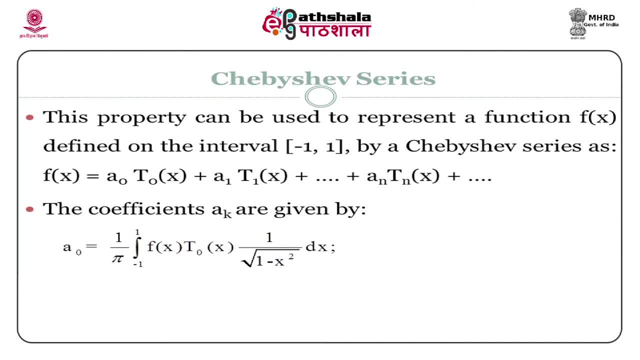 integral and use orthogonal property. So only one first term will survive and all other terms will die out or will be 0 and therefore a 0 will be given by 1 upon pi minus 1 to 1, f, x into t 0, x into 1 upon n root of 1 minus x square dx, because this side will be t 0. 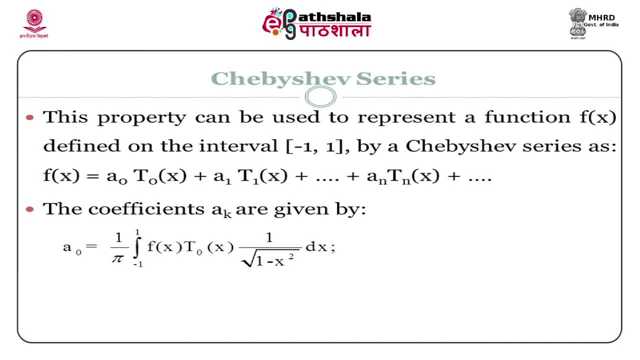 x square and that will be pi, and that will have to take it on the other side. So 1 upon pi into minus 1 to 1 f x. So this will be t 0 x square and that will be pi, and that will. 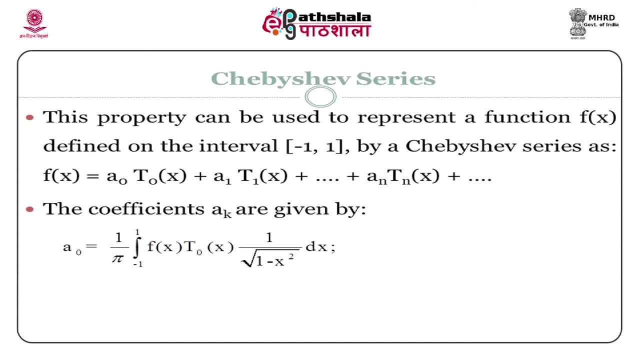 be pi and that will have to take it on the other side. So 1 upon pi into minus 1 to 1, f, x into t, 0, x upon 1. n. root of 1 minus root. square root of 1 minus x, square dx is a 0. 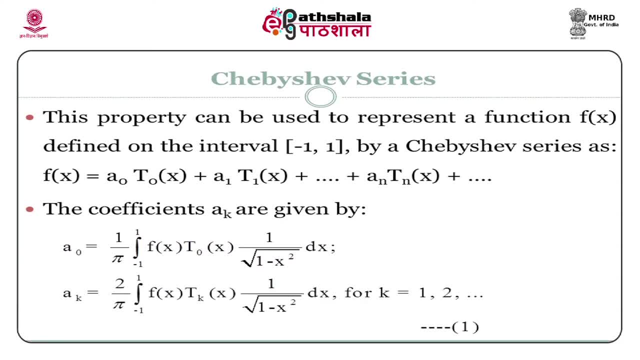 and similarly a k will be given by 2, by pi minus 1 to 1, f, x into t, k, x upon into 1 upon n, root of 1 minus x square dx. So for k equal to 1,, 2, 3 onwards, this formula will be valid. 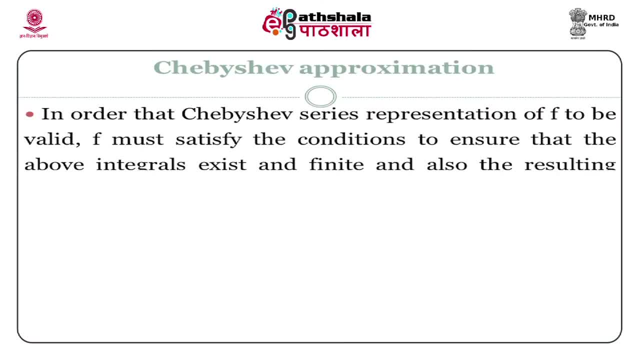 and that gives me the Chebyshev series. In order that the Chebyshev series, representation of f, to be valid, f must satisfy the conditions to ensure that the above integrals exist and finite, So the resulting series must converge. Existence is necessary, without which we cannot write. 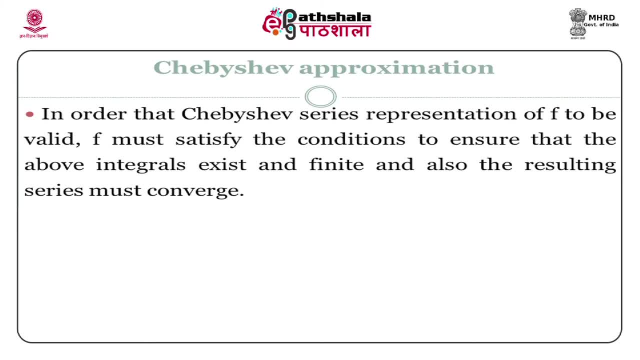 down those integrals, and finiteness is necessary because each term has to be finite, otherwise we cannot add, and also the resulting entire series must converge in order to this series representation to be valid. In case when the series converges, f can be approximated by nth degree polynomial given. 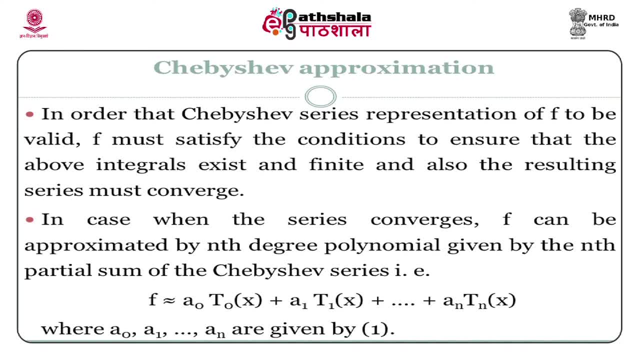 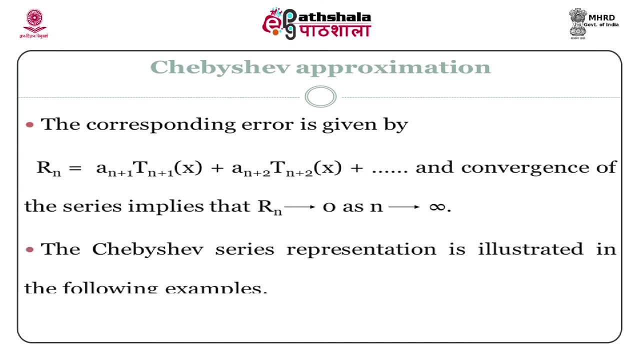 by the nth partial sum of the Chebyshev series, and f can be approximated like this by a0t0x plus ntnx, where these are given by formulae discussed earlier in 1.. The corresponding error is given by Rn equal to n plus 1 tn plus 1 x plus n plus 2 tn plus 2 x, and so on. Convergence: 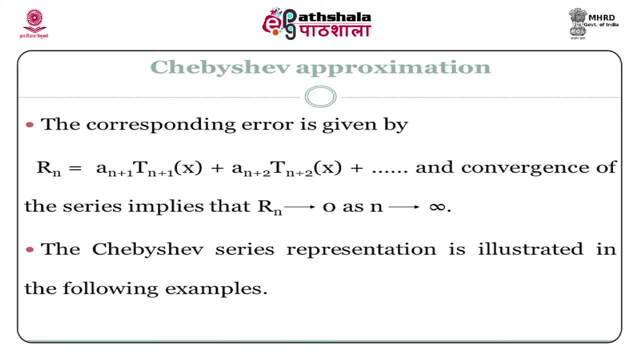 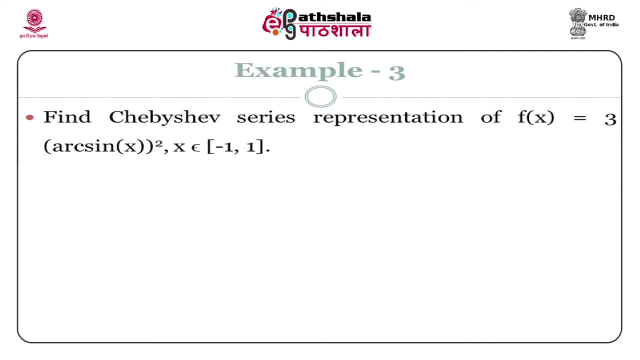 of the series implies that this Rn tends to 0 as n tends to infinity. Now this example 3 gives me fine Chebyshev series representation of f, x equal to 3 into arc sin x, whole square x belonging to minus 1 to 1.. So by 1 we will get a0, 1 upon pi. 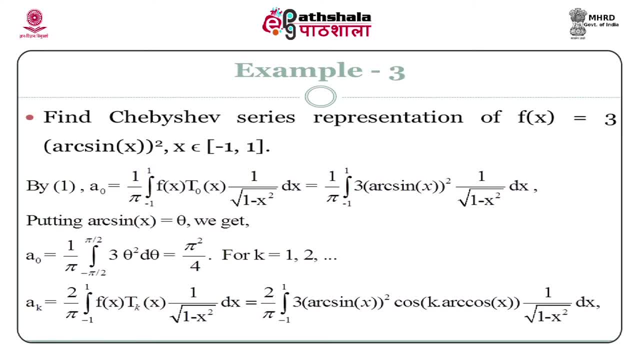 into minus 1 to 1, f x into t0 x, 1 upon n root of 1 minus x square dx equal to 1 upon pi. into minus 1 to 1, 3 into arc sin x whole square. into 1 upon n root of 1 minus 1 plus x square. 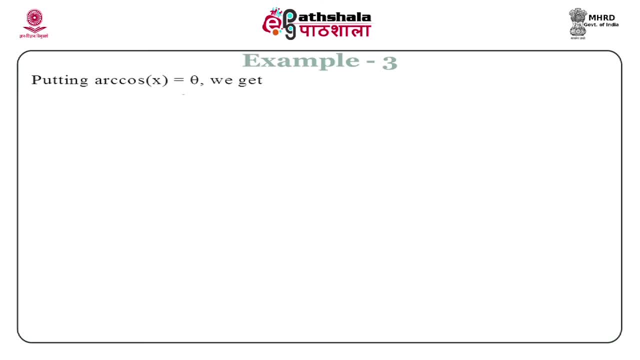 root 1 minus x square dx. Putting arc sin x equal to 0, we get a0 equal to 1 upon pi minus pi by 2 to pi by 2, 3 theta, square d theta which gives me pi square by 4 for k equal. 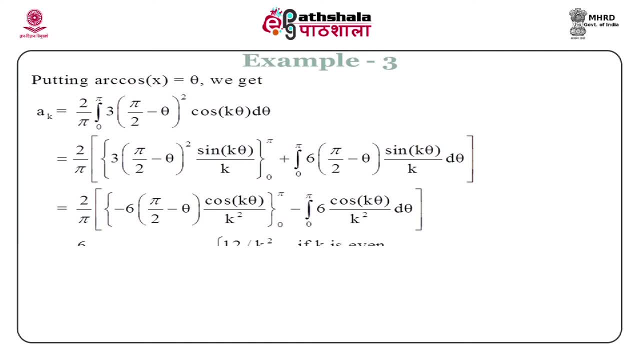 to 1.. So this is for a0, x, For k equal to 1,, 2 and 3.. In other words, if I put f, x is equal to 3- into arc sin x square, I will get this integral. 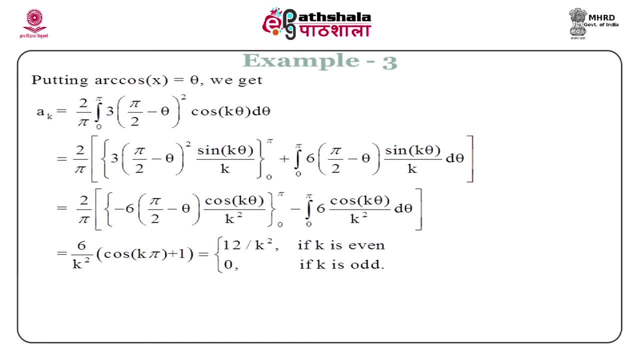 ak as 2 by pi minus 1 to 1, 3 arc sin x whole square into cos k. r cos x upon into 1 upon n root of 1 minus x square dx. Again I put this value putting r cos x equal to theta. 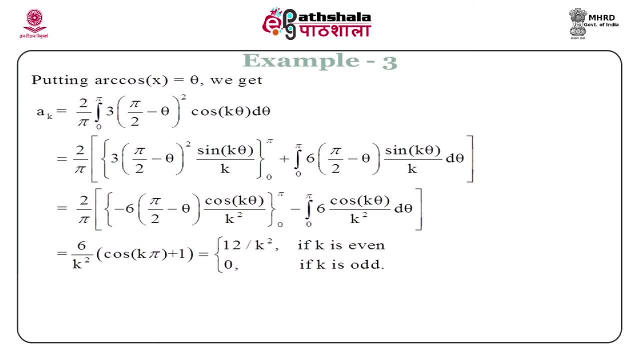 I will get this as 2 by pi 3 into pi by 2 minus theta, whole square into cos k, theta d theta, And if I integrate it by parts, finally I will get this: integral will be equal to 12 by k square if k is even and 0 if k is odd. So thus ak will be equal to 12 by k. 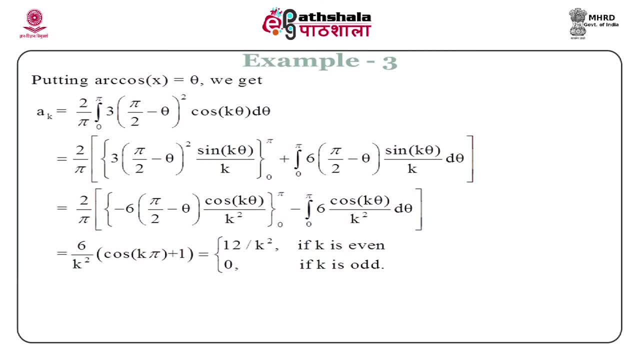 square if k is even and 0 if k is odd. So thus Chebyshev series expansion of f is given by pi square by 4, into t 0 x plus 3, into 1 upon 1 square, into t 2 x plus 1 upon 2 square. 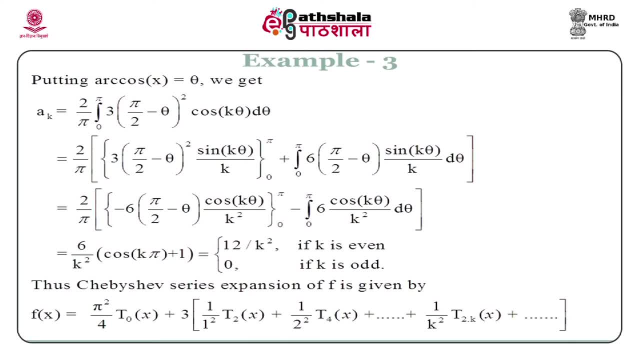 into t 4 x and so on. In general term will be 1 upon k square into t 2 k x. So we have seen here that ak is given by 12 by k square if k is even and 0 if k is odd. So this is: 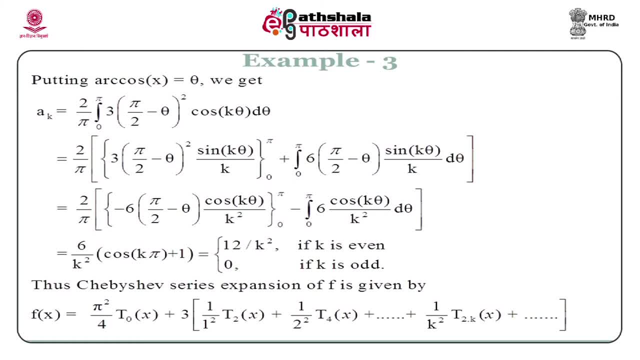 very simple. Thus the Chebyshev series expansion of f is given by f x equal to pi square by 4, into t 0 x plus 3, into bracket 1 upon 1 square t 2 x plus 1 upon 2 square t 4 x plus so on. 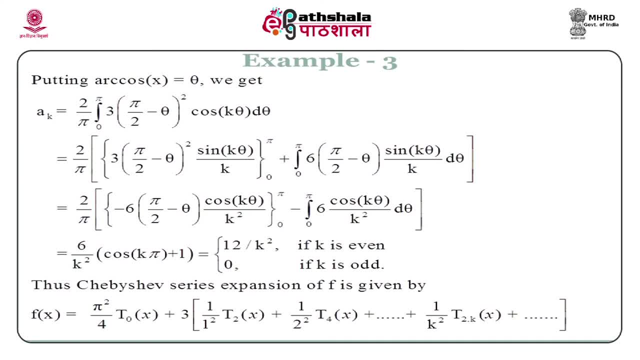 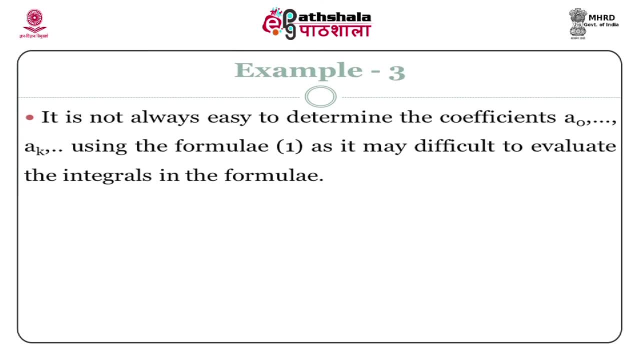 1 upon k square into t, 2, k, x plus so on. It is not always easy to determine the coefficients a 0, a k using the formula 1, as it may be difficult to evaluate the integrals in the formulae For some function whose Maclaurin series expansion. 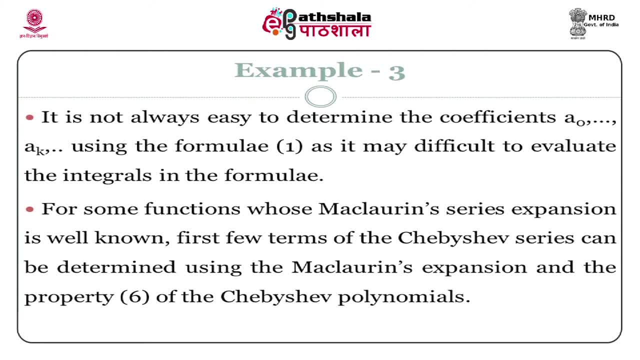 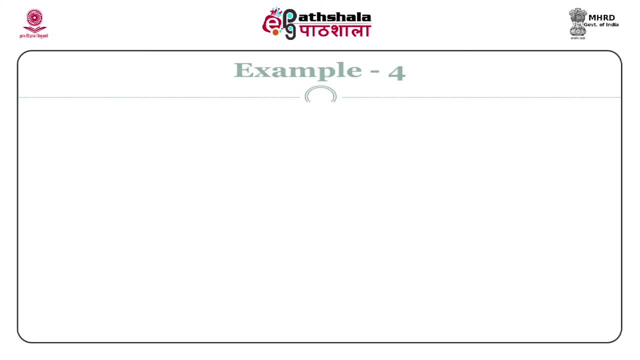 is well known, first few terms of the Chebyshev series can be determined using Maclaurin's expansion and the property 6 of the Chebyshev polynomial. This is illustrated in the following example 4, which says that determine the first few. 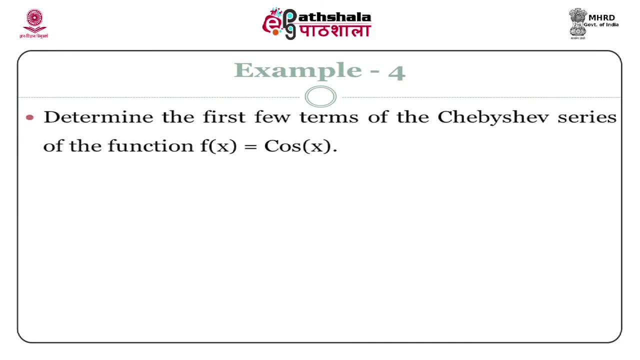 terms of the Chebyshev series of the function f? x equal to cos x. The Maclaurin series, expansion of f? x is given by cos x equal to 1 minus x, square by 2, factorial plus x less to 4, by. 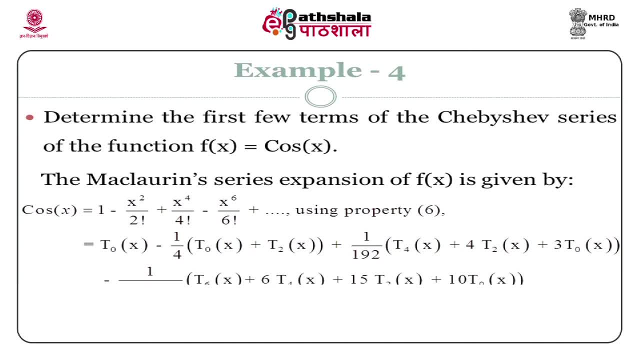 4 factorial. x raise to 6 by 6 minus x raise to 6 by 6, factorial, and so on. Now, using property 6, we will express this: x square, x raise to 4, x raise to 6 in terms of Chebyshev. 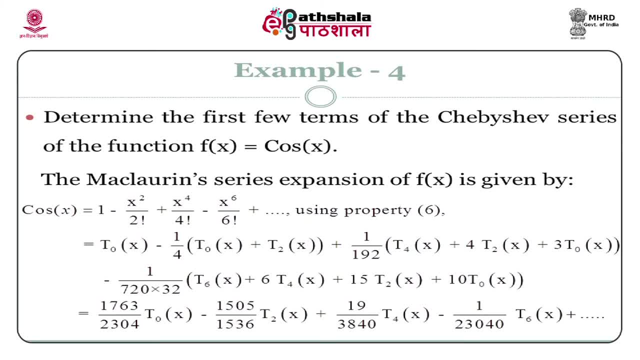 polynomials and therefore we can see that we get cos x equal to t 0 x minus 1 by 4 into bracket t 0 x plus t 2 x plus 1 upon 1, 9, 2 into t 4 x plus 4. t 2 x plus 3 into t 0 x. 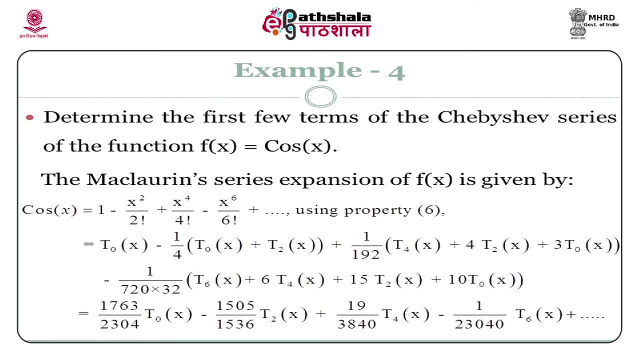 minus 1 upon 7 20 into 32, into t 6 x plus 6 t 4 x plus 15 t 2 x plus 10 t 0 x, and then on, On simplification, we will get the corresponding few. first four terms of the this Chebyshev. 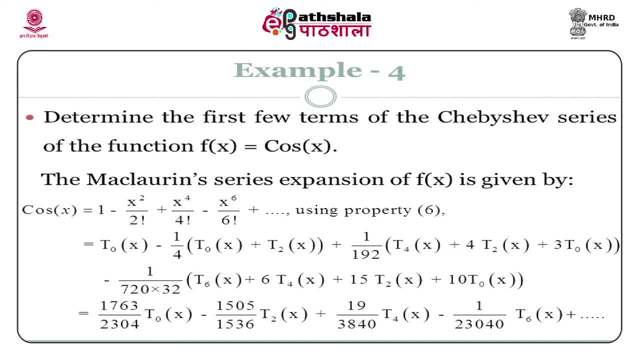 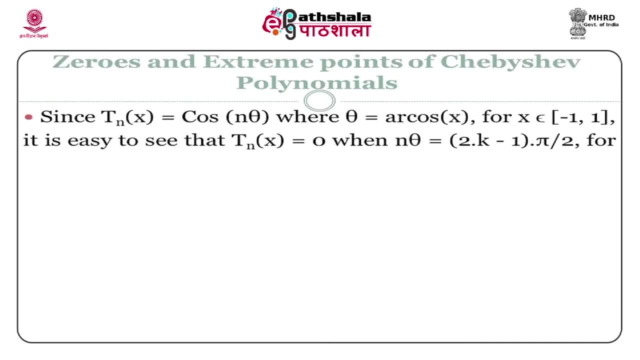 series for this function. Now we are going to talk about one of the important properties of the Chebyshev polynomials, and for that we will be discussing what are the zeros and extreme points of the Chebyshev polynomial. Now, since t n, x is equal to cos n, theta, where 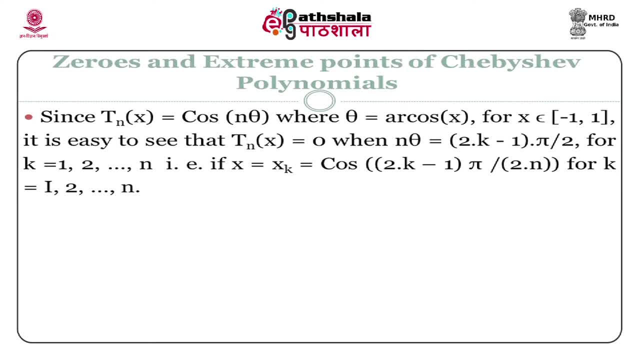 theta is r cos x for x belonging to minus 1 to 1, it is easy to see that t n x equal to 0 when n theta is 0. So t n x is equal to 2 into k minus 1, pi by 2 for k equal to 1 to 3, and so on That. 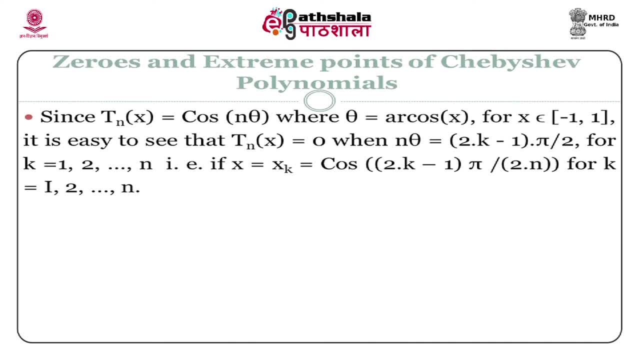 is: if x equal to x k, which is given by cos of 2 k minus 1, pi by 2 n for k equal to 1 to 3 up to n. So we can see here that n theta equal to this. therefore theta equal to this. 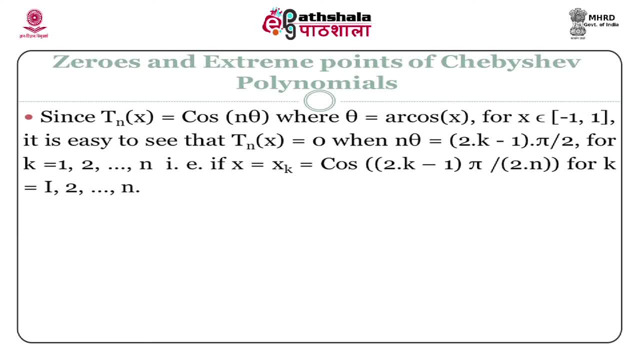 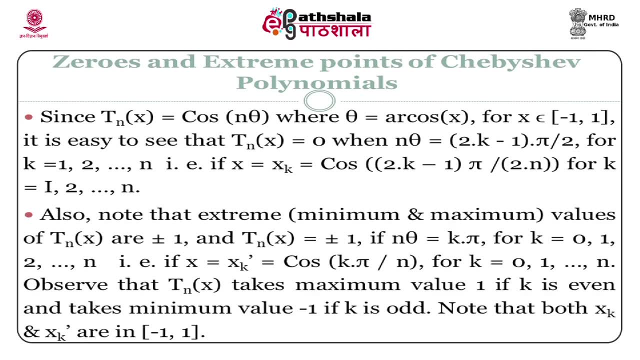 and then theta is nothing, but x is equal to cos theta and therefore we get x equal to x, k as the zeros of this polynomial t n x. Also, note that the extreme point or extreme values, that is, minimum and maximum values of t n x are plus or minus 1 because, being a cos n theta, and these are attained at t. 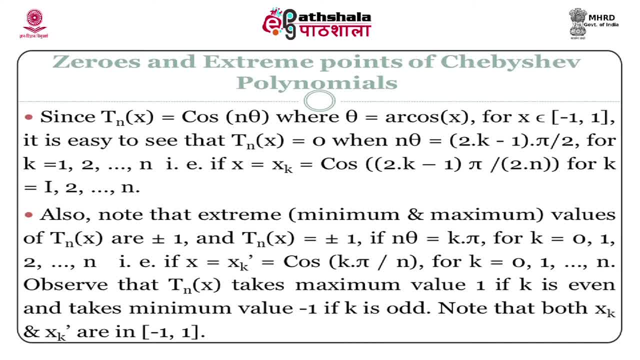 n. x equal to plus or minus 1. if n theta is equal to k, pi for k equal to 0, 1 to 3 up to n. That is, if x equal to x, k which is equal to cos of k, pi by n for k equal to 0, 1 to. 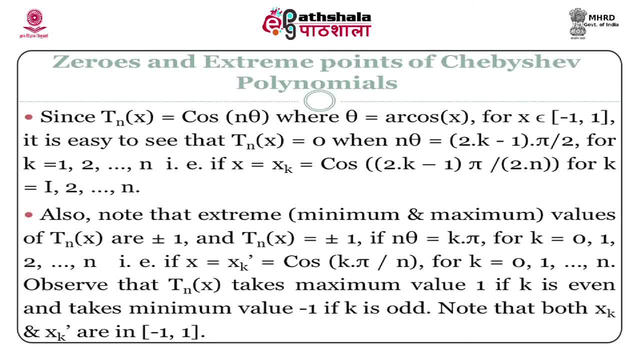 3 up to n. Observe that t n x takes minimum value 1 if k is even and takes maximum value 1, if k is even and takes minimum value minus 1 if k is odd, Note that both extreme points x- k and x k dash are in minus 1 to 1.. So here extreme points are denoted by x k dash. 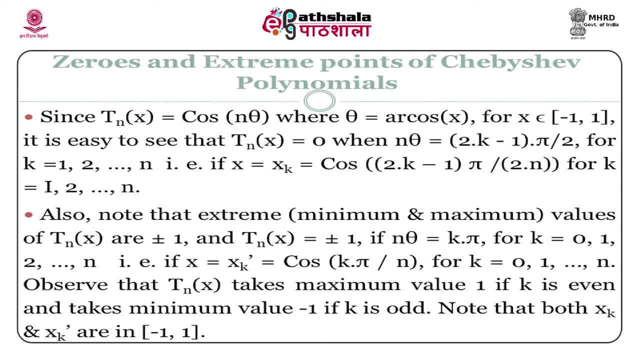 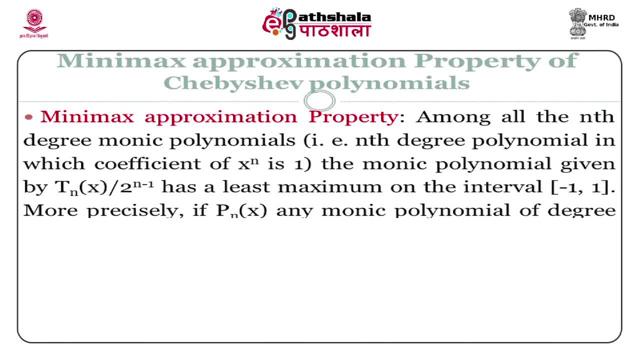 and the zeros are denoted by x, k, and all of them are in minus 1 to 1.. So minimax approximation property we are talking about. So, among all the monic polynomials, the monic polynomial given by t, n, x upon 2 raise to n minus 1, has a least maximum on the interval minus 1 to. 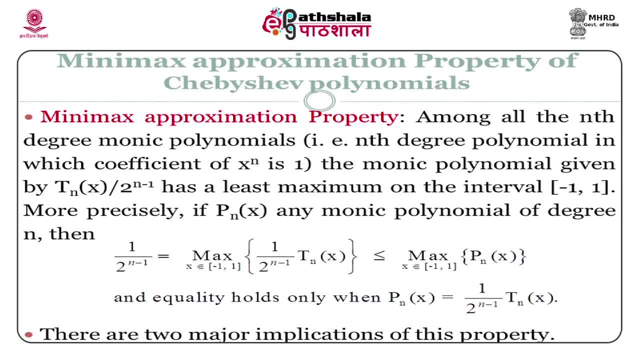 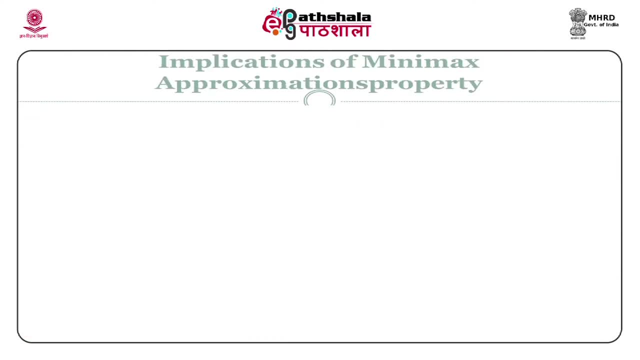 1. As long as p, n, x is any monic polynomial, then 1 upon 2 raise to n minus 1 is equal to maximum. of is more closely than the green curve, which is the Lagrangian interpolating polynomial on arbitrary nodes, Also using the same property for reducing the degree. 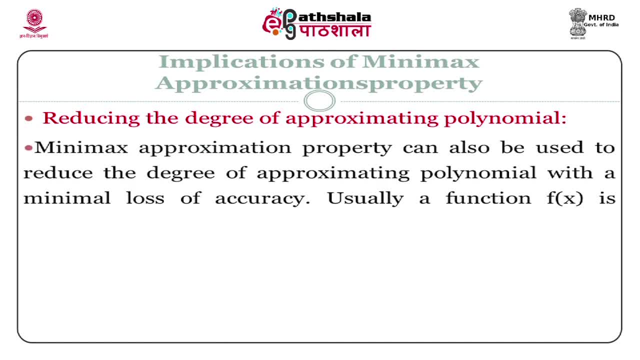 of approximating polynomial. so minimax approximation property can also be used to reduce the degree of approximating polynomial with a minimal loss of accuracy. Usually a function f, x is approximated by a Taylor's or Maclaurin's polynomial of some degree. n As n increases. 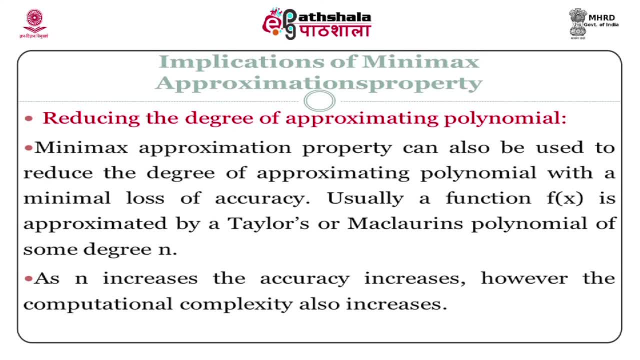 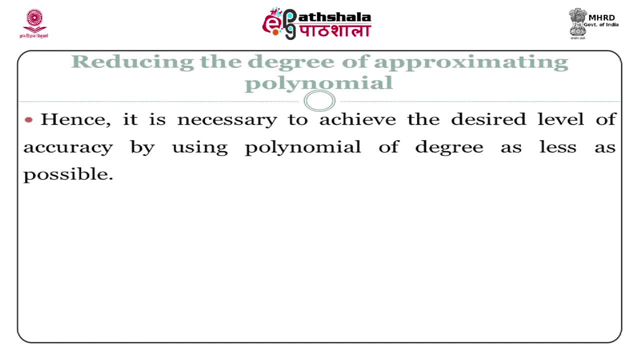 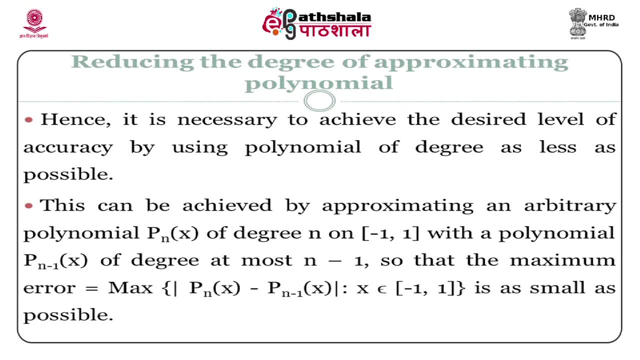 the accuracy increases, However, the computational complexity also increases. Hence it is necessary to achieve the desired level of accuracy by using polynomial of degree as less as possible. This can be achieved by approximating an arbitrary polynomial Pn x of degree n on minus 1 to 1 with a polynomial of Pn minus 1 of degree at most n minus 1. 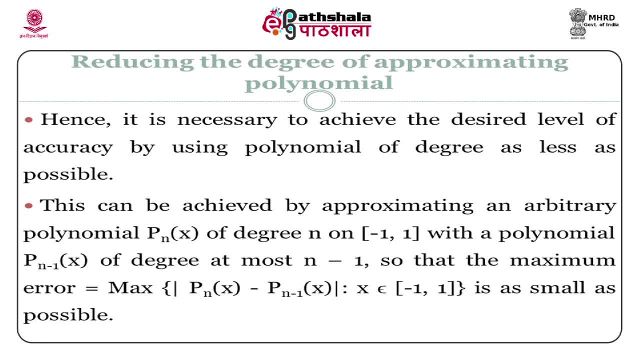 polynomial Pn minus 1, x of degree, at most n minus 1,, so that the maximum error equal to maximum Pn x minus Pn minus 1 x x belonging to minus 1 to 1 is as small as possible. So. 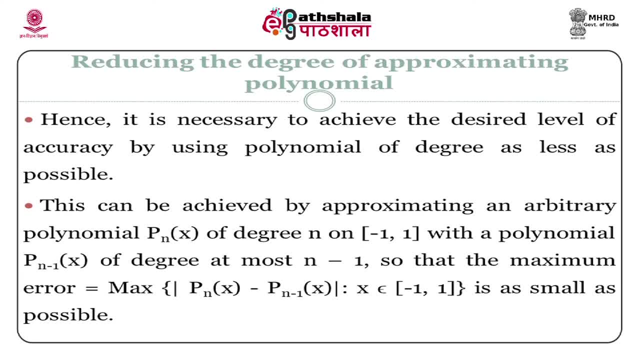 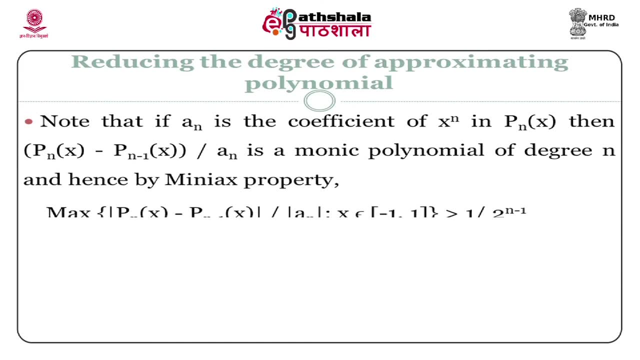 that means difference between the nth degree polynomial approximation and n minus 1 degree polynomial approximation. So difference between these polynomials should also be minimized. maximum difference also should be minimized. So note that if a, n is the coefficient of x, raise to n in Pn x, then Pn x minus Pn minus. 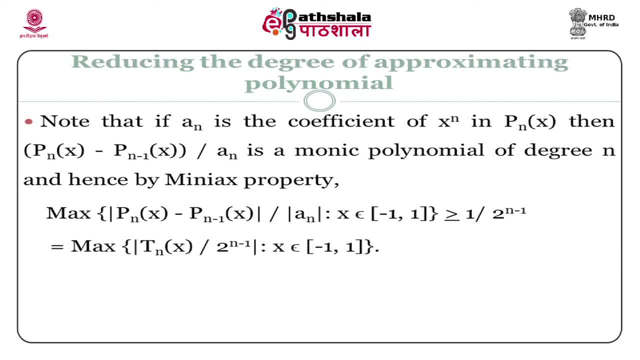 1- x divided by a n is monic polynomial of degree n And hence by minimax property, maximum value of Pn x minus Pn minus 1 x divided by mod a- n, the interval minus 1 to 1, which 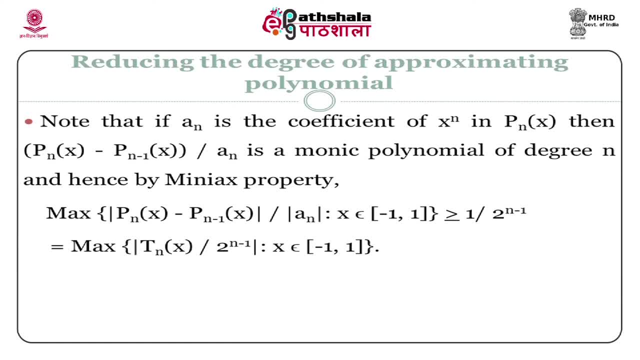 is going to be greater than equal to 1, upon 2, raise to n minus 1, and which is equal to maximum of Tn minus 1.. Thus, if we take Pn minus 1, x minus Pn x, as Pn x minus a n into Tn x by 2, the desired 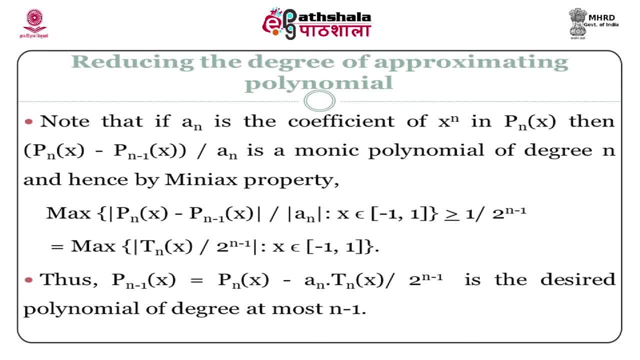 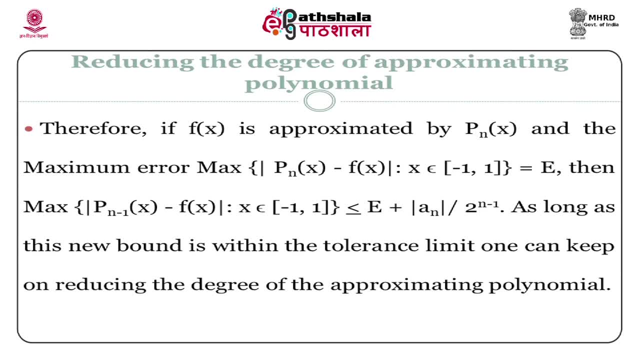 polynomial of degree, at most n minus 1 can be obtained. Therefore, if f x is approximated by Pn x and the maximum error max of mod Pn x minus f x or x minus x belonging to minus 1 to 1 is equal to e, 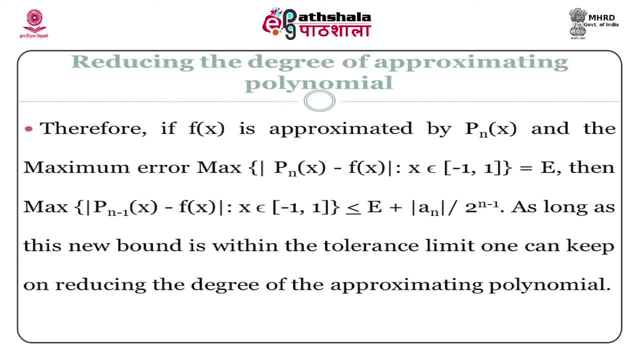 The maximum error between Pn minus 1 x and f x is going to be, at most e plus mod a, n by 2 raise to n minus 1.. As long as this new bound is within the tolerance limit, one can keep on reducing the degree of the approximating polynomial. So therefore, if f x is approximated, 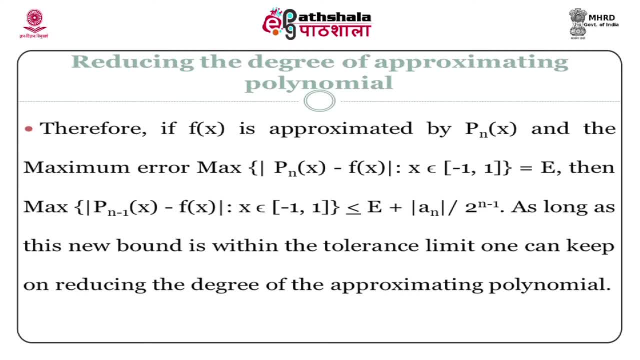 by Pn x and the maximum error max of mod Pn x minus f x. x belonging to minus 1 to 1 is equal to e. Then we can also make the special rule sacred to the headまた. x is reduced by Pn x and. 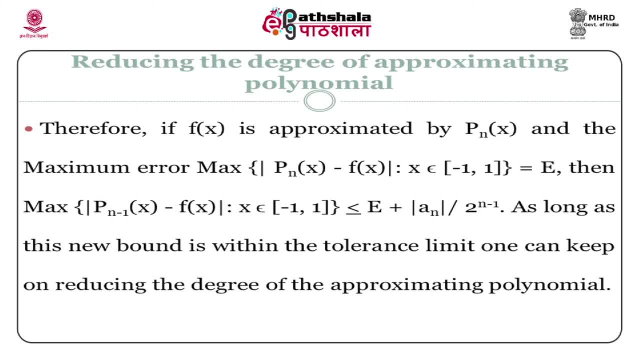 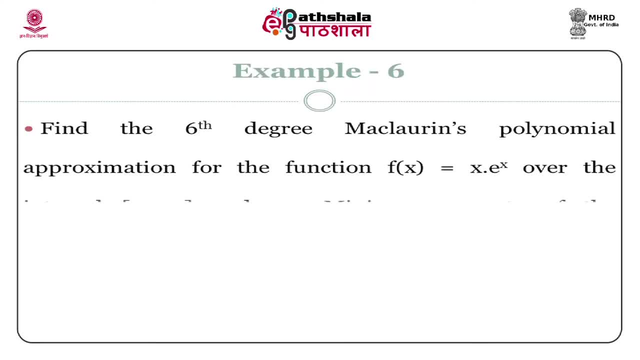 x ts belonging to dean x and x loss from n. That is the 완� Architect configurationук for any x related to snap initial needed linear vertex And if I have to assume this feature, I can simply state that this日本 constraint. 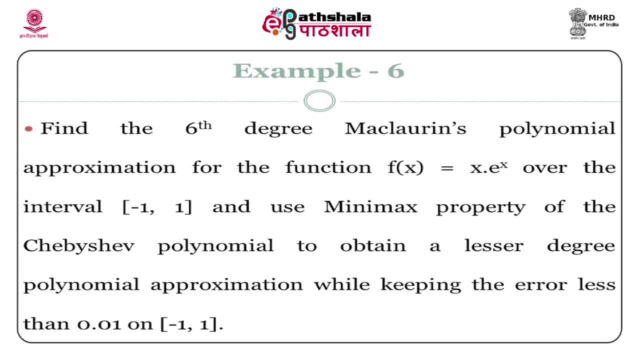 is diferentes for x, z and x as an interpolation, income for T over tribute to n minus 1, minus f, x, x over the interval minus 1 to 1, and use minimax property of the Chebyshev polynomial to obtain a lesser degree polynomial approximation while keeping the error less than 0.01 on minus. 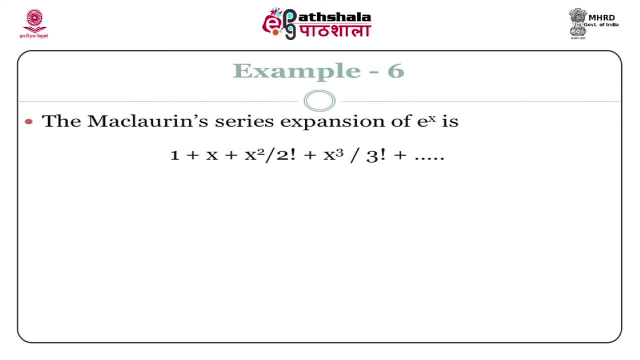 1 to 1.. The Maclaurin series expansion of e raised to x is 1 plus x plus x square by 2 factorial, plus x cube by 3 factorial, and so on, and hence the 6 degree Maclaurin's polynomial approximation. 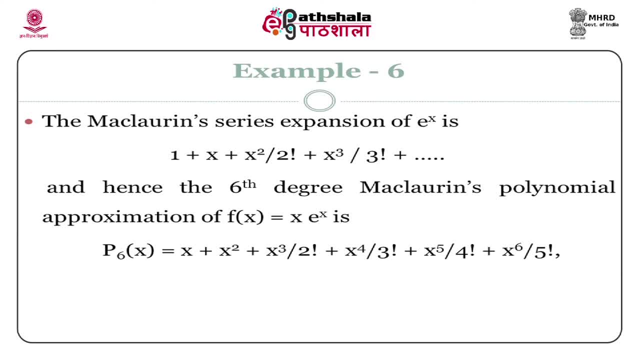 of x, e raised to x is going to be given by p: 6, x equal to x, x square, x cube by 3 factorial, plus x raised to 4 by 3 factorial plus x raised to 5 by 4 factorial, and x raised to 6 by 5. 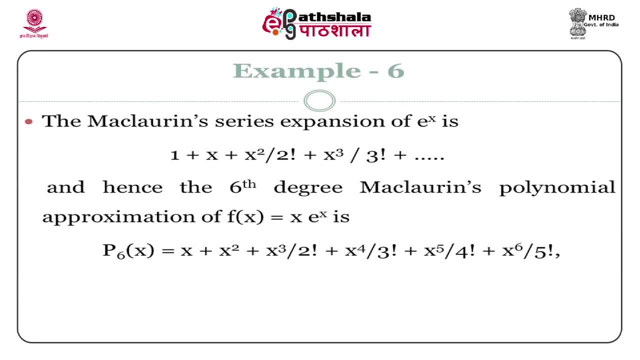 factorial. So we are using Maclaurin series expansion of e raised to x to get Maclaurin series expansion of x into e raised to x and the truncation error R 6, x will be given by e, c, x, e raised. 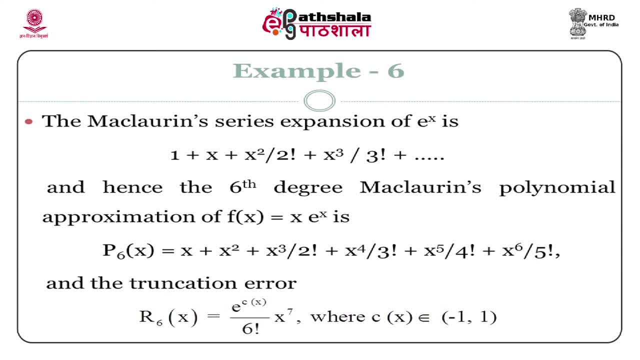 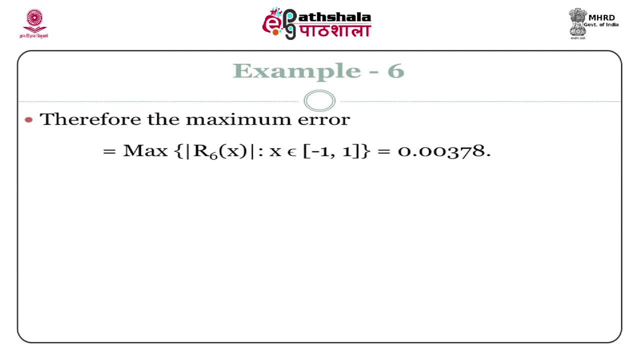 to c x upon 6 factorial into x raised to 7, where c x is in some point in minus 1 to 1.. Therefore, the maximum error that is maximum for mod R, 6 x, x belonging to minus 1 to 1. 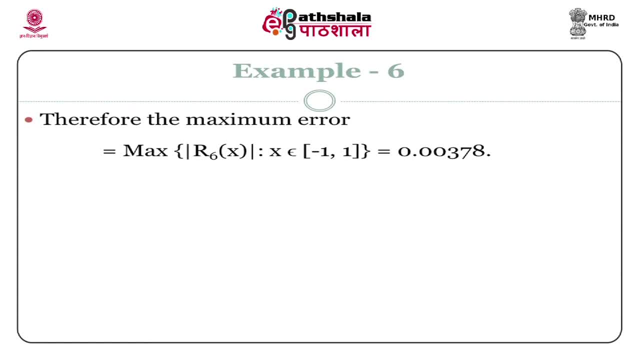 will be roughly 0.00378.. Now reducing the degree of approximating polynomial by procedure I had discussed above. what we will have to do is see what we need is the approximation error. we want it to be less than 0.01.. 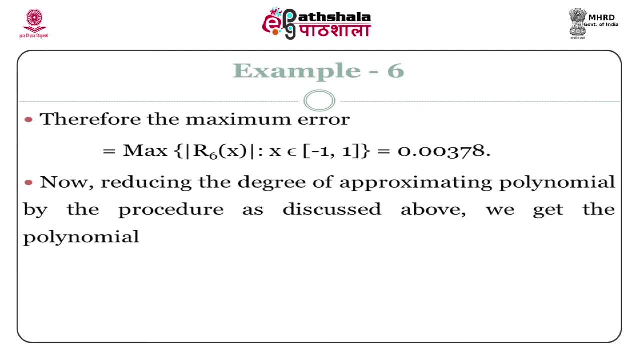 So our tolerance limit is up to 0.01, whereas here we have got error 0.00378.. So 0.00378.. So error is too small as compared to the tolerance limit, and hence we have a scope. 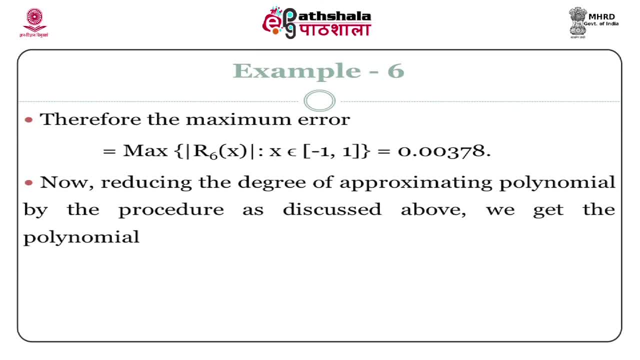 to reduce the degree of approximating polynomial. So following that procedure we are doing now, p 5 x will be taking as p 6 x minus 1 upon 5 factorial into t 6 x divided by 2 raised to 5.. 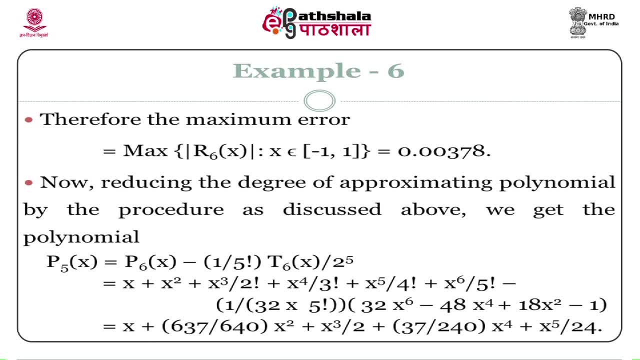 So we will be considering here 1 upon 5 factorial into t 6 x, like that we are considering and therefore we will get the polynomial approximation like this: So p 6 x minus 1 upon 5 factorial into 2 raised to 6 x divided by 2 raised to 5.. 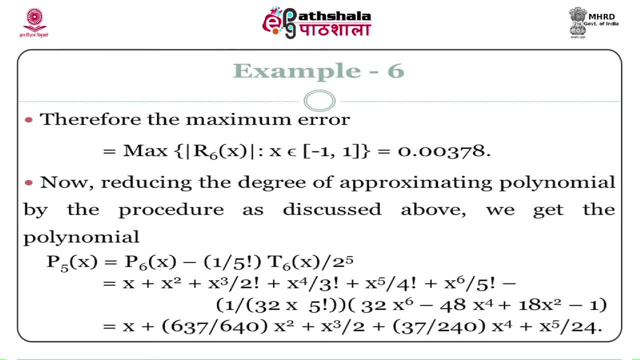 So x plus x square plus x cube by 2 factorial, which is plus x raised to 4 by 3 factorial plus x raised to 5 by 4 factorial, plus x raised to 6 by 5 factorial minus, we get 1 upon 32. 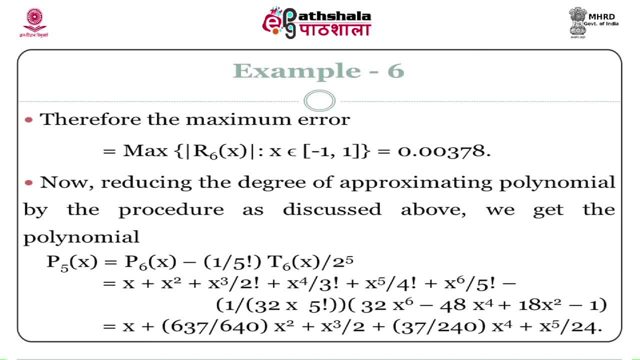 into 5 factorial, into t 6 x, which is given to be 32 x raised to 6 minus 48 x raised to 4 plus 18 x square minus 1.. And that gives me the polynomial like this: x plus 6, 37 by 6, 40 x square plus x cube by. 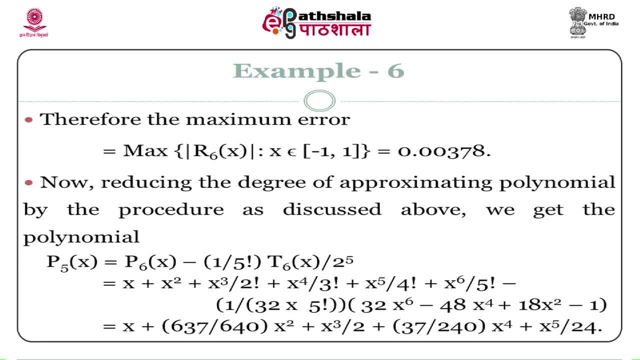 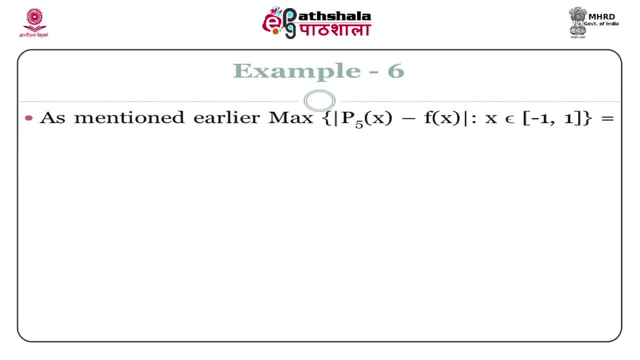 2. 37 by 240 into x, raise to 4 plus x, raise to 5 by 24.. So this is your P5x we get and, as mentioned earlier, maximum error between P5x and Fx will be equal to the earlier error. 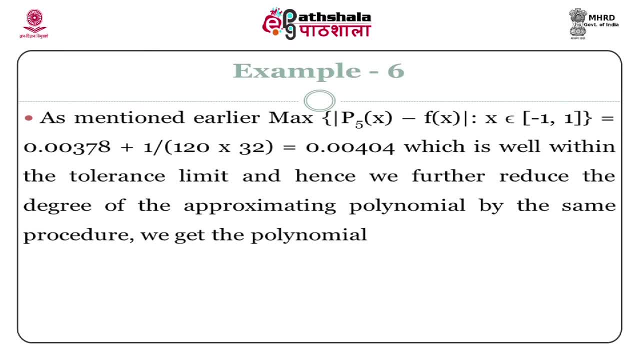 that is E 0.00378 plus 1 upon 120 into 32, and therefore the total of that error will be 0.00404, which is well within the tolerance limit, and hence we can further reduce the degree of the approximating polynomial. So now again we are taking P4x as P5x minus. 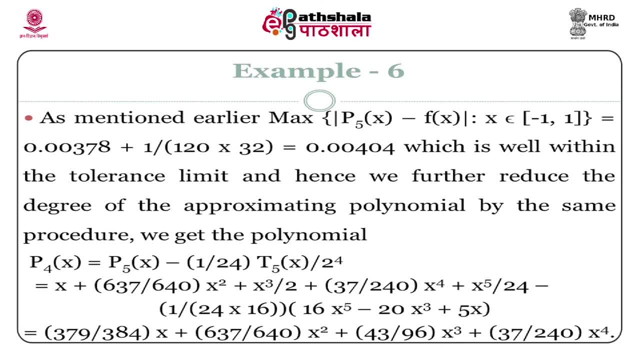 1 upon 24 into T5x, divided by 2, raise to 4 and on simplification we get. So we get P4x as 379 by 384 x plus 637 by 640 x square, plus 43 by 96 x cube, plus 37 by 240 x raise to. 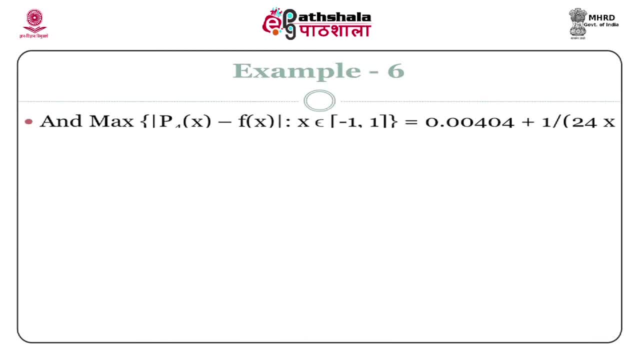 4. And the maximum error, that is P4x minus Fx, over the interval minus 1 to 1, will be given by earlier error, 0.00404 plus 1 upon 24 into 16, that is equal to totaling that I will get. 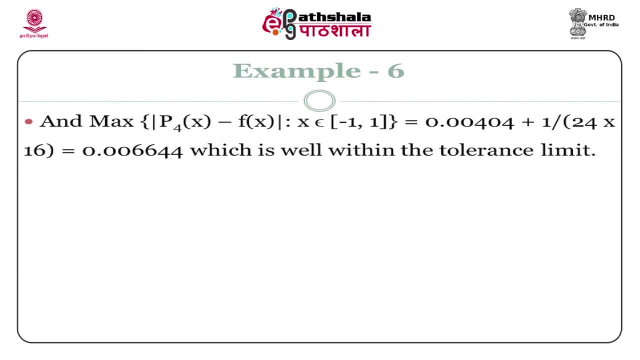 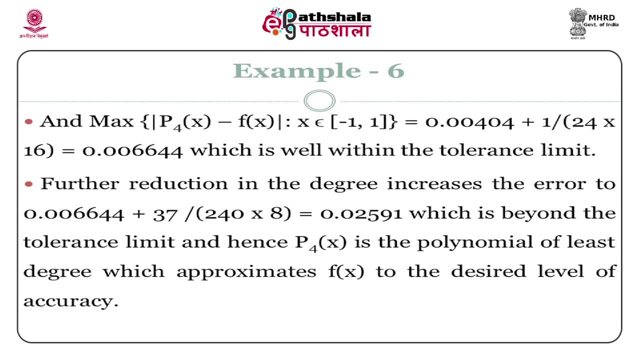 0.006644, which is well within the tolerance limit. Further reduction, if we do in the degree, increases the error to 0.006644, plus 37 by 384 x, square divided by 240 into 8, and that will give me error 0.02591, which is beyond the tolerance. 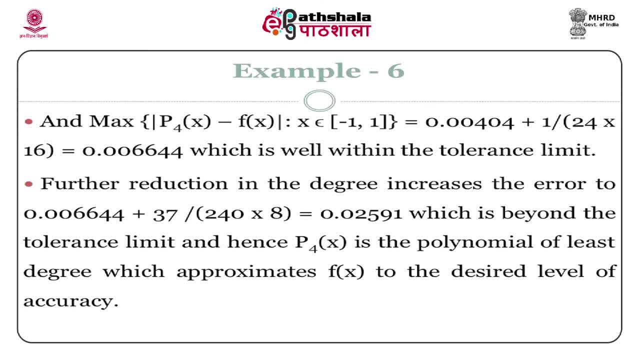 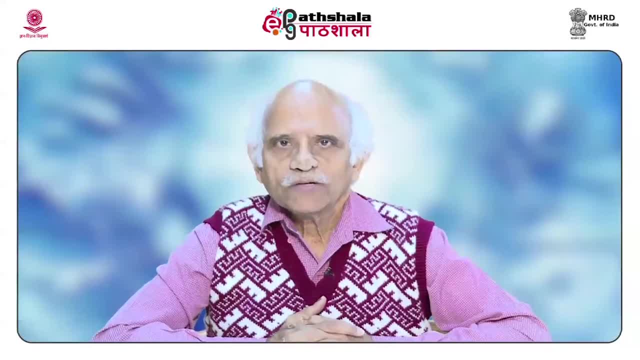 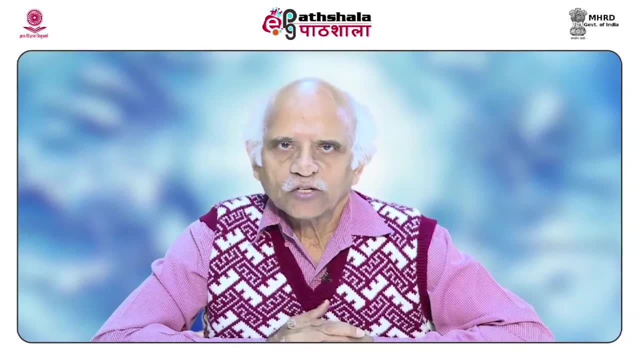 limit, and hence P4x is the polynomial of least degree which approximates Fx to the desired level of accuracy. In this module we have seen the methods for approximating function which are other than interpolation and curve fitting. Here we are using two techniques for function approximation. 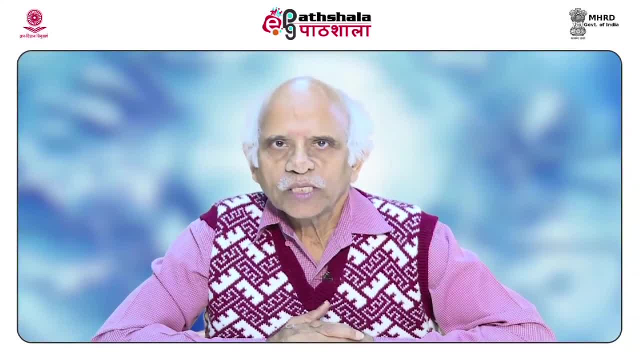 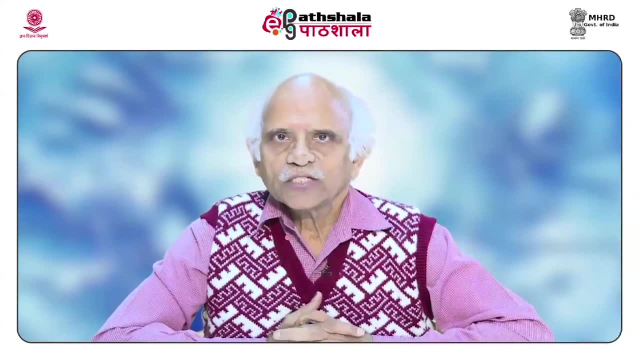 One Taylor's polynomial or Mc laurin's polynomial and the second Chebyshev polynomials are used for function approximation. In the first case we get Taylor's or Mc laurin's series approximation and the truncation error Rn. we could find out from that. 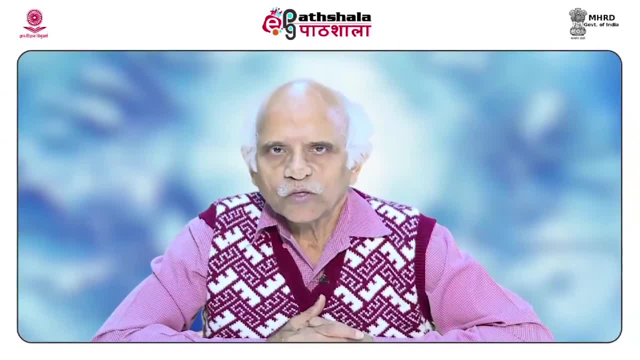 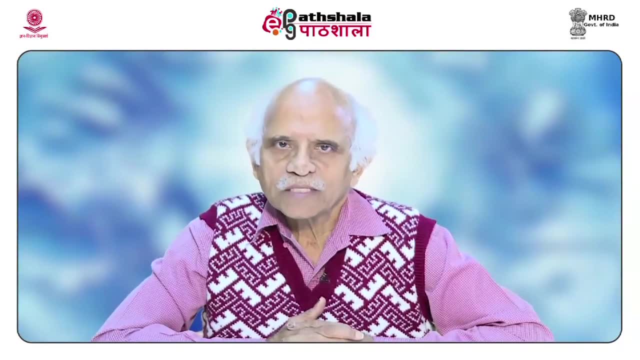 In the second for Chebyshev polynomials. we have to introduce Chebyshev polynomials. we introduced that and we have seen several properties of the Chebyshev polynomials. One of the important properties of a mini max polynomial property we have considered. 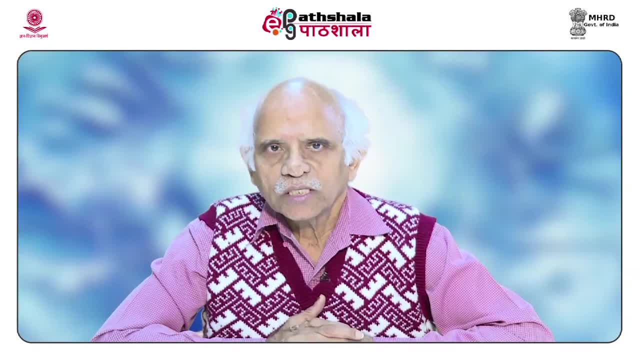 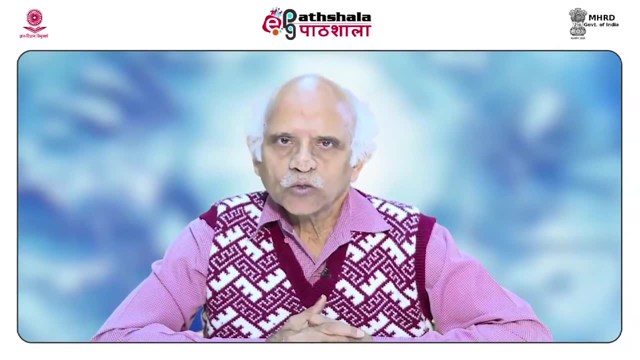 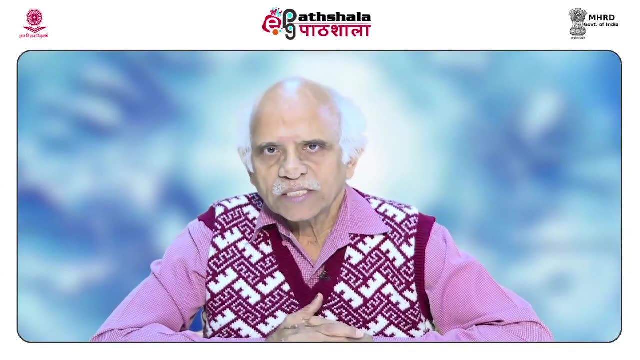 for Chebyshev polynomial polynomials and its implication in reducing the interpolation error is being illustrated by giving certain examples. and also that minimax property has been used to reduce the degree of approximating polynomial is being used. Thus, in this particular module we have seen the techniques for function approximation. 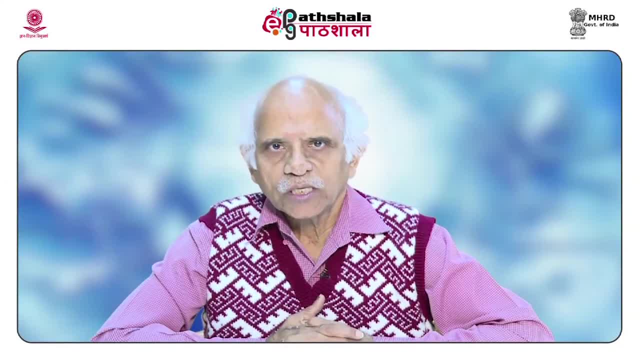 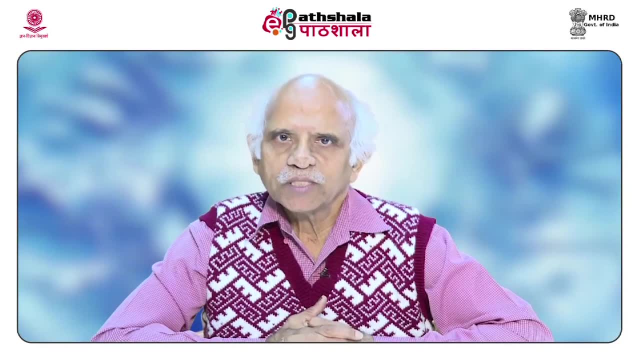 and their implications on reduction of error in the interpolation and their implications on reducing the degree of approximating polynomial has been illustrated.